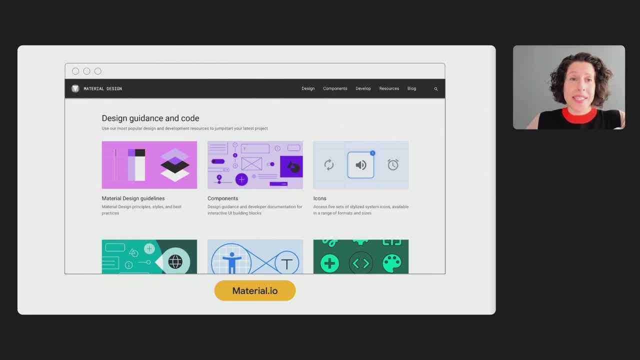 build high-quality digital experience. You might have even seen it mentioned in the keynote yesterday Where we announced Material U, So the communication section covers a lot more than UX writing. There are topics ranging from data visualization to onboarding to empty state patterns, And I recommend you. 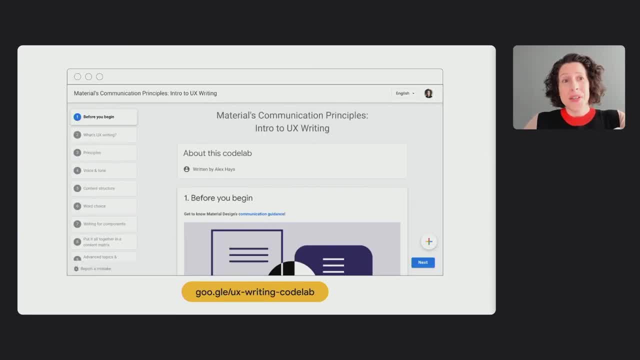 check it out. Now let's talk writing. So today's workshop is set up based on a code lab And they're designed to walk you through new skill or experience, And the link at the bottom of the screen in my slide takes you through the process of writing a new skill. 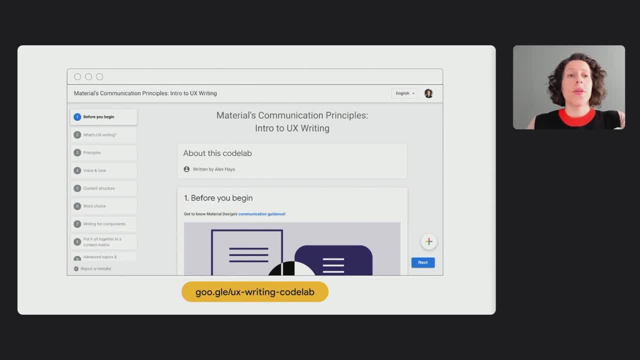 So let's get started. takes you to the workshop, and there should also be a link in the workshop player. You don't need to go there now to participate, but you can if you want to. My slides will repeat the same content in the code lab, so you can just focus on this window for the hour if you want. 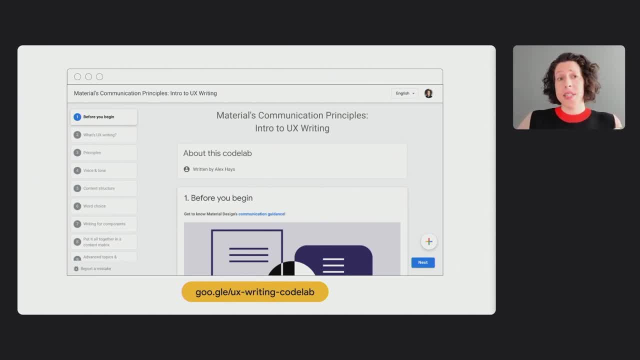 You can go back to the code lab later and see the lessons in depth if you're interested in trying out some more exercises, and it also works with your own content. So I'll keep that link up for a second and a little more setup and we'll be on our way. 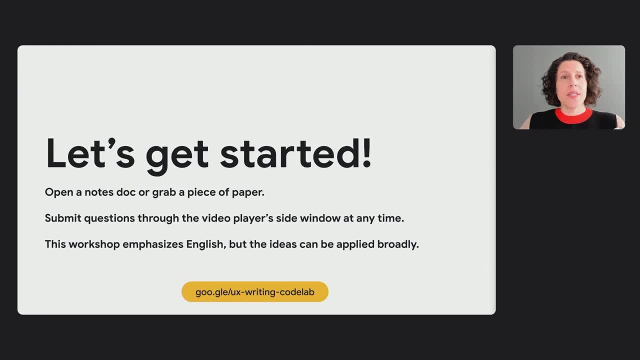 So there should be a panel alongside this video and it's for Q&A. You can submit any questions in there and it will be live for 12 more hours after the workshop. And lastly, I want to mention that I'm thrilled IO has such a huge global audience this year. 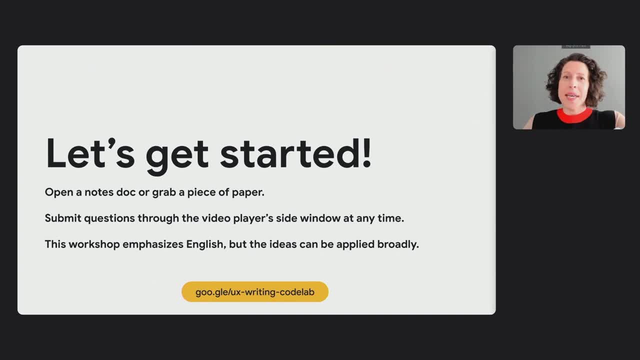 It's great to be virtual And I want to mention that because this is the first time that I've had a virtual workshop. So I'm really excited to be here And I want to mention that because this is the first time that I've had a virtual workshop. 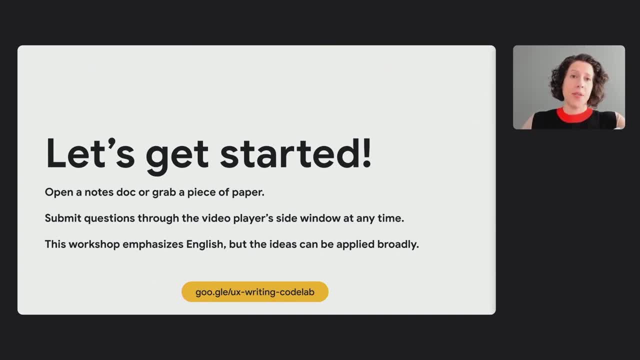 And I want to mention that because this is the first time that I've had a virtual workshop. This lab covers communication principles for better user experiences, But in reality, it's really about American English. That's what I'm fluent in, And the examples and word choices are based on conventions of American English. 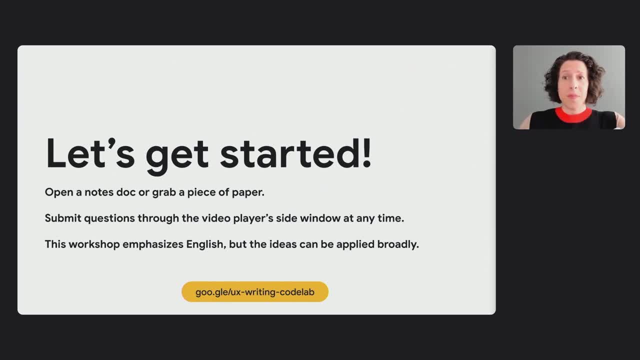 So I want to say that up front, but also recognize that there's a lot of multilingual designers in the audience today. So, with sensitivity to changes in context and culture, I think you can use a lot of this information in any UI. I also want to mention that 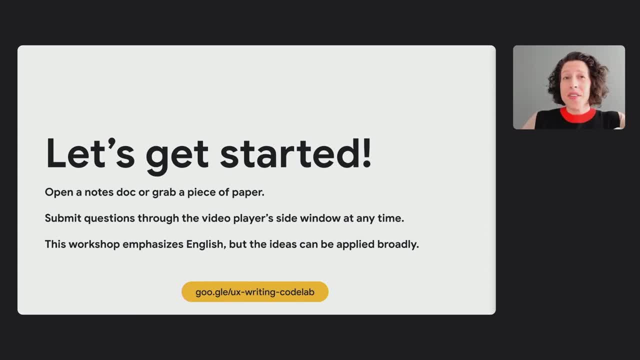 my colleague and teammate has created a lot of great resources on global writing. They're linked from the code lab and can help you work through some of those specifics too. So, if you can't tell already, I love being a writer on the UX team at Google. 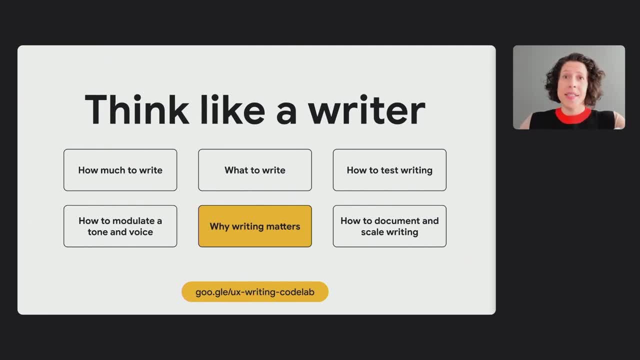 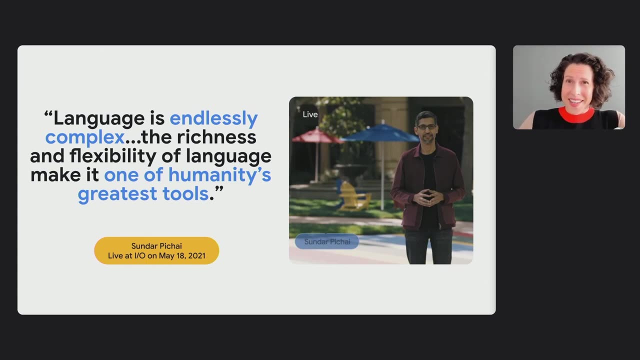 We'll talk a little bit about what a UX writer does and what questions writers ask, And hopefully through that you can see why language matters in product experiences. I can understand if you're thinking: I don't need to think like a writer, I think like me. 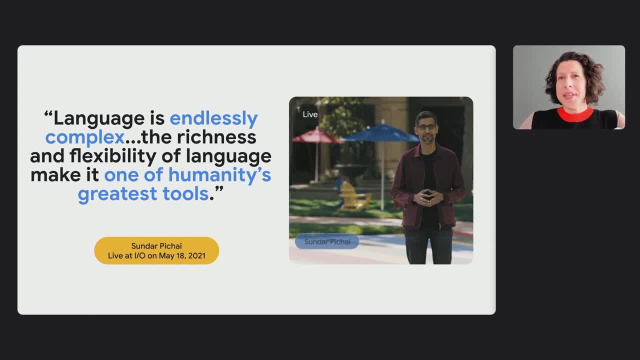 And I do different work. And didn't Sindar say yesterday in the keynote that writing is obsolete now? anyways, with advances in natural language understanding? Well, sort of. So his words were: language is endlessly complex. The richness and flexibility of language makes it one of humanity's greatest tools. So it's a little different, And 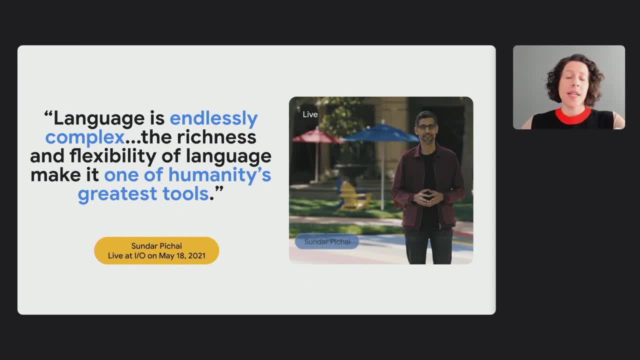 what I hear there is that it's a tool, and that's a lot of the definition of UX, writing being goal-oriented, and that it's complex, which is also why we're here right now to make sense of it together, And my own belief is that writing is a critical piece of system thinking, which is why 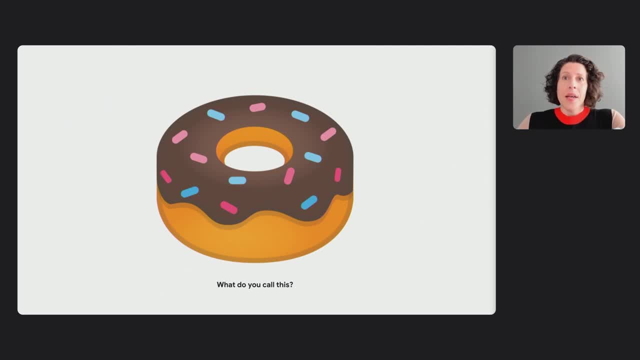 it's part of material design. So maybe another example, not from quantum computing, but everyday communication, will also help make my case. So this is a quiz for you. What do you call this? Let you think of the name, And if we were live together, I might name a few terms. 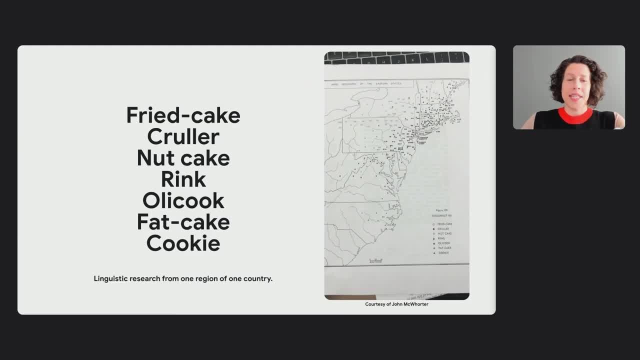 see whose hand is raised. but I'll jump straight to the case Within this map that I received from John McWhorter. it shows linguistic research from one region of the United States might use all of these terms. So that's one country and one region. I say donut, but you know. 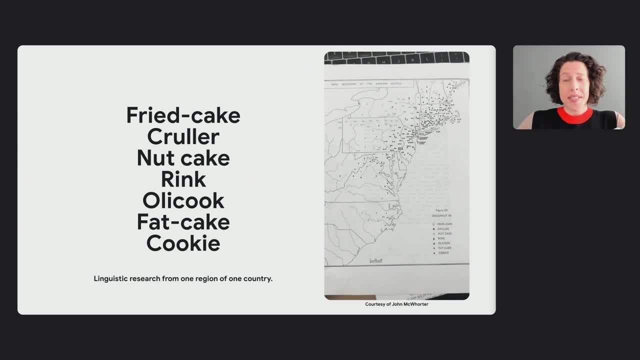 we have global users And if we were to take research from the United States, from one region, we might use all the terms, So that's one country and one region. I say doughnut, but we have global users, And, And creating clear experiences for any person is no simple feat, when you think about just how subjective our expressions are. 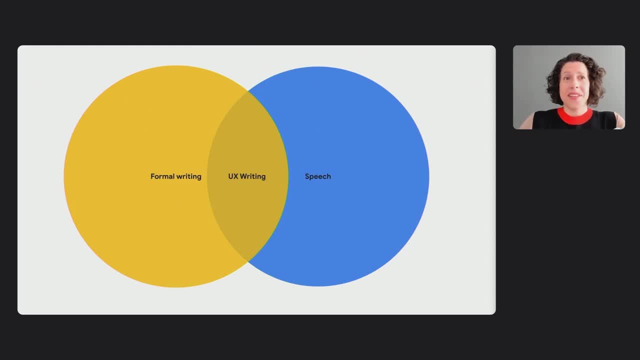 And that's also what makes it exciting: Language is never stable and a writer's work is never done. UX writing combines the academic rules of formal writing- So the stuff you read in a newspaper, or nonfiction books- with the less formal styles that people use when communicating online. 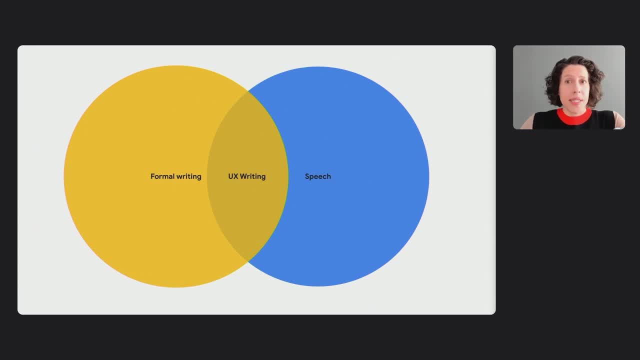 Email text, chat. So writing for apps and interfaces takes a less formal tone for two main reasons. Online communication tends towards less formal than printer academic writing And UI text is limited by screen. real estate Character length is always constrained, So where does that leave us? 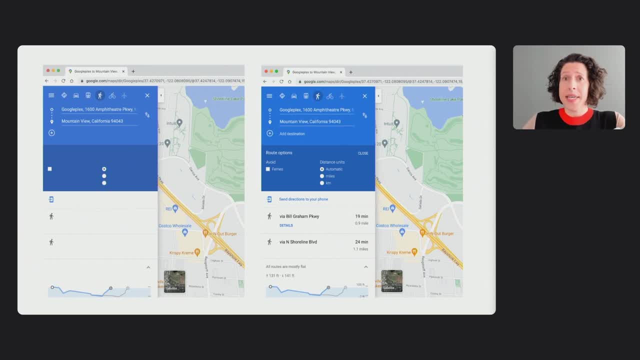 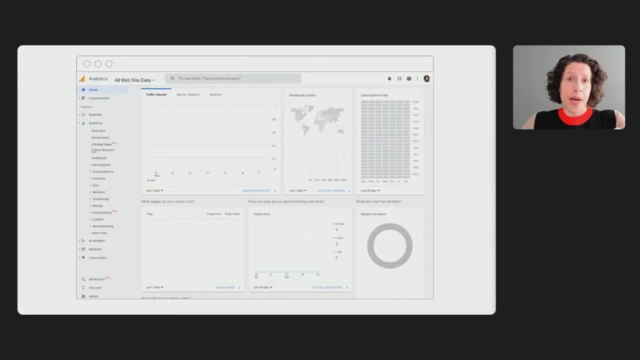 Well, what I do know is that without writing, we'd be lost. The UI. text, in every form, plays an essential role in the quality of user experiences. It's all over the UI. Most teams don't have writers. It's often done by designers, engineers or PMs. 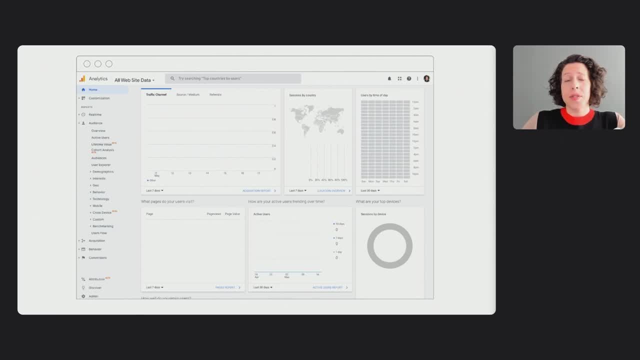 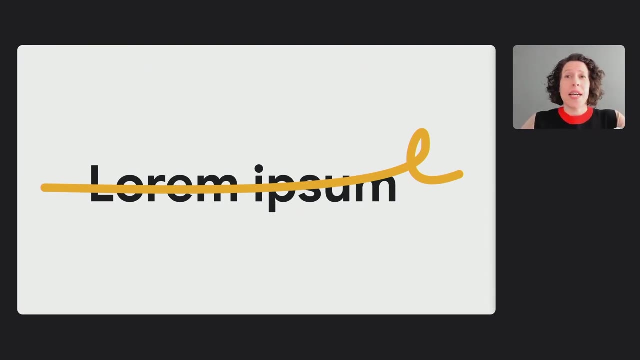 So really that means that everyone should build an awareness of the role language plays in delivering good experiences. Otherwise, it could end up more like this. That would be really hard to use. And if you remember one thing from today, I want to emphasize that UX writing is about goals and interactions. 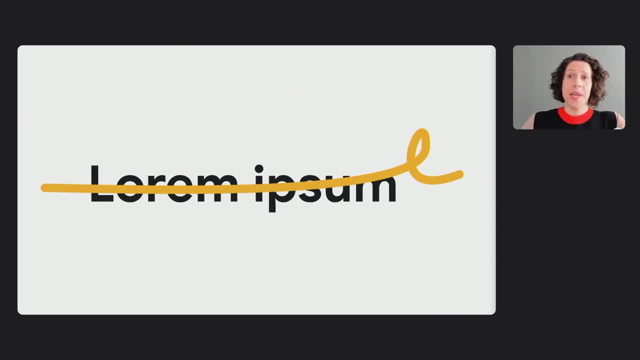 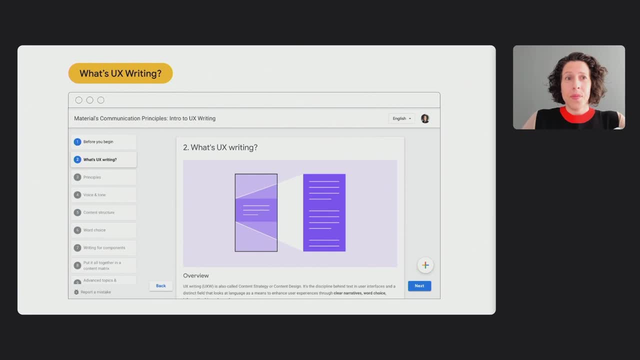 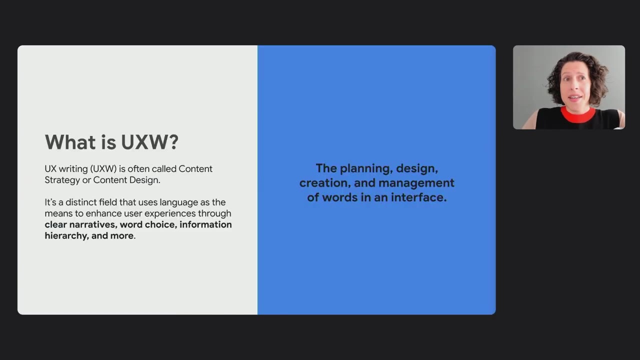 So using real words and not filler text like lorem ipsum in the context of your writing. So if you're in the code lab, we're on to step two now, where we get into what is UX writing. First of all, UX writing is a UX discipline. 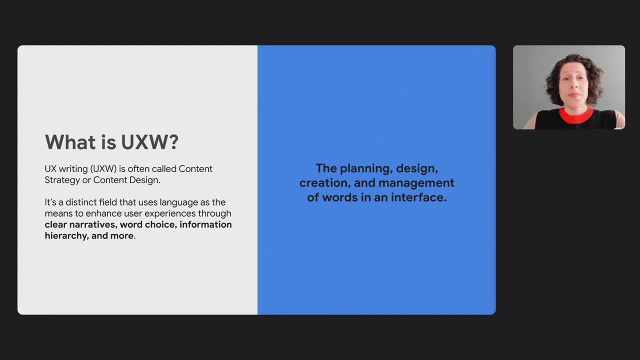 It's distinct from tech, writing, copywriting and marketing. In short, it's the planning, design, creation and management of words in an interface. I also want to mention that you might hear the terms content strategist or content designer around. 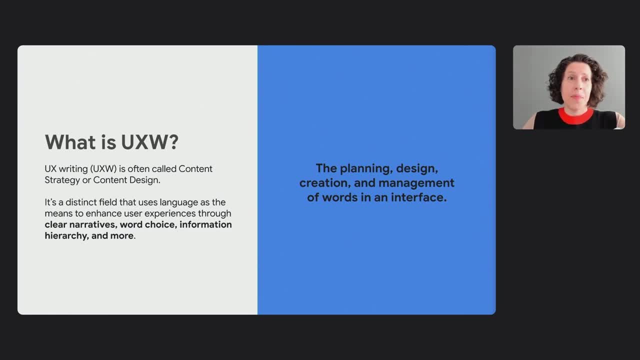 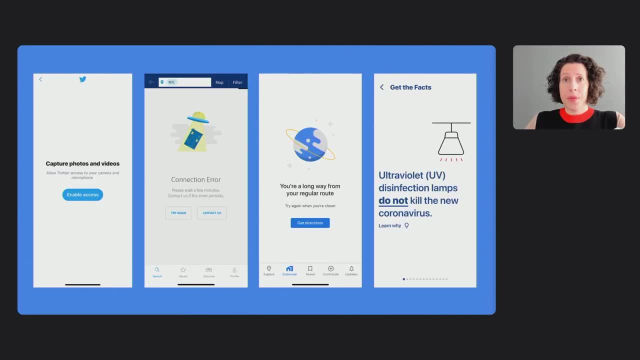 And that's pretty similar. The point is that people with those titles are looking at the narratives, word choice, information hierarchy and more, So here's some examples of what we usually think of as UX writing. A lot of the time we think of it as the fun stuff, the jokes and animations that abound. 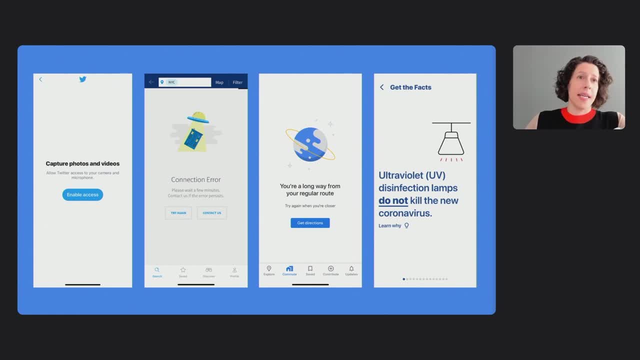 It's that casual, fun tech voice, But there's actually a lot at stake. Words: when they fill empty spaces, they really enhance task completion, User satisfaction and overall ease of use. On the far right, that's actually an app I worked on last year. 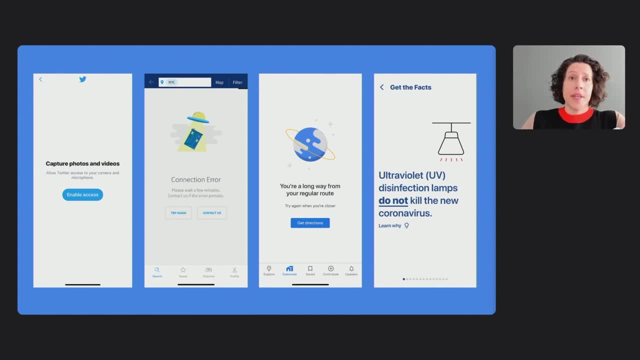 It was a collaboration with the World Health Organization and the Flutter team here at Google, And in the case of a COVID app, there's serious consequences. You don't always want it to be like a joke or leave any ambiguity, really, when we're talking about a global pandemic. 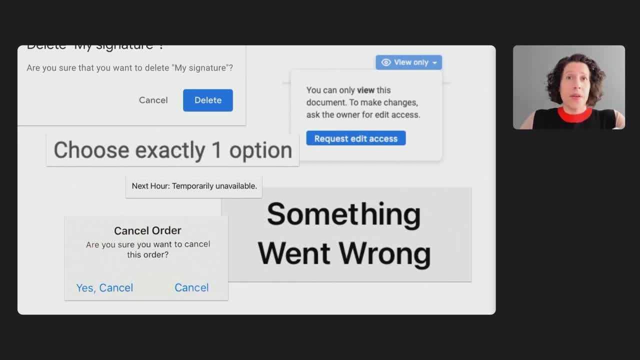 And when things do go wrong, the right words and tones are critical. That example in the bottom left that says cancel order has two actions that all say cancel. I feel like that's something we're going to get to later- why you really need to pay attention to each label in the context of everything around it. 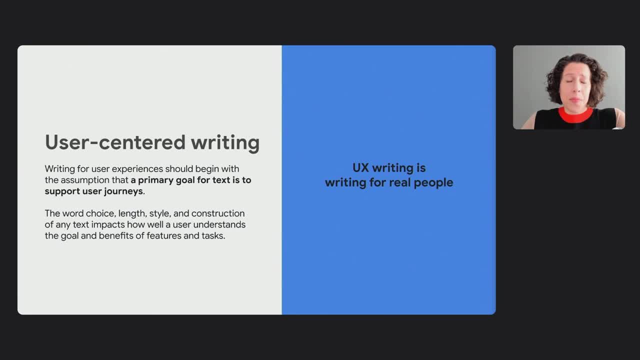 So UX writing is user-centered writing. It's writing for real people, And that's because the primary goal for text is to support user journeys. The word choice, length, style and constructiveness of the text are important, And the direction of text impacts how well the user understands the goals and benefits of your features and tasks. 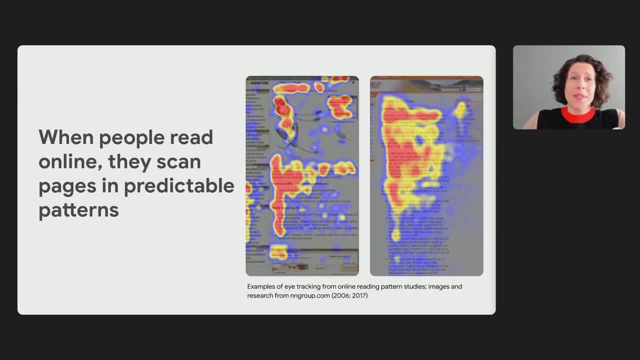 And to write means to consider how people read This one's important, So you might have seen this before. This is some great research from Nielsen Norman Group. It was done in 2006 and then repeated with the same results in 2017.. 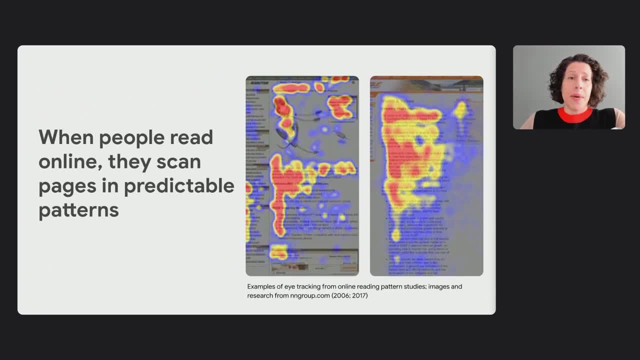 It shows that when people read, they scan images in predictable patterns. This heat map shows an F-shaped pattern, But again, the important word here is scan. People scan. They don't read every word you write, So that means that we really have to use short paragraphs. 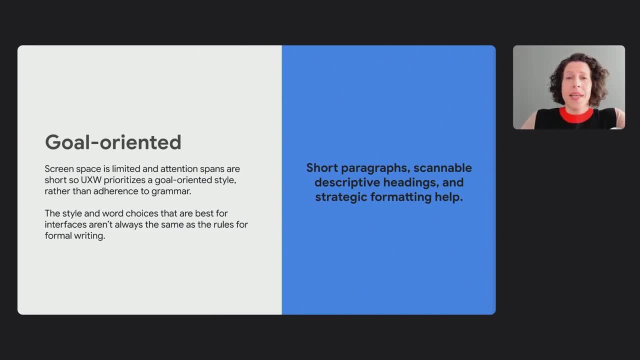 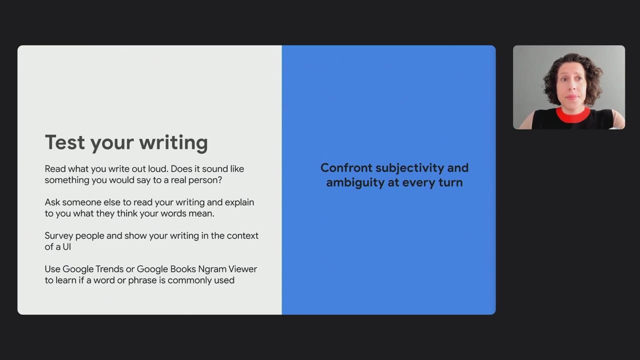 scannable descriptive headings and strategic formatting. It's goal-oriented writing, So that means that we have to choose between adherence to grammar versus what gets your user from point A to point B, And if UX writing is all about meeting your goals. 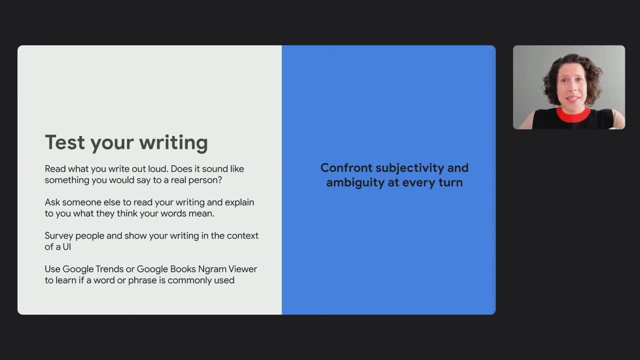 how do you know if you've met them? That's where testing comes in, So it's important that you try any method that's available to you. On this slide, I'm showing some of the easy, more affordable, often free methods. 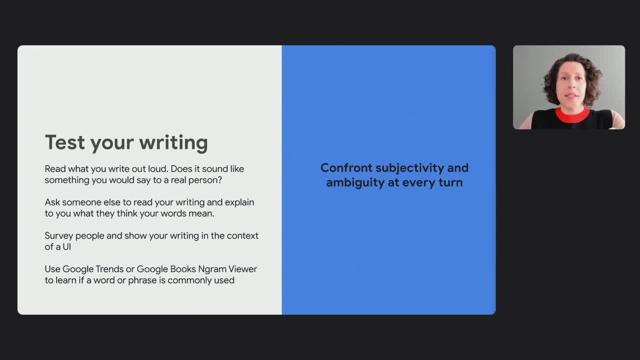 And it's a way of just confronting the inherent subjectivity in language. So what I like to do at the most basic level is read things out loud. Would I say this to a friend? If not, I should probably rewrite it, And that's it. 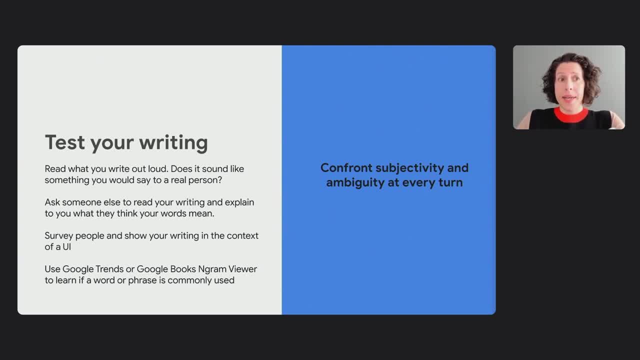 And I can ask someone else to read my writing and explain what they think I said. Another option is to always show the writing in the context of a UI. Tools like Google Trends or the Google Books Ngram viewer is a way of seeing if a word choice is common. 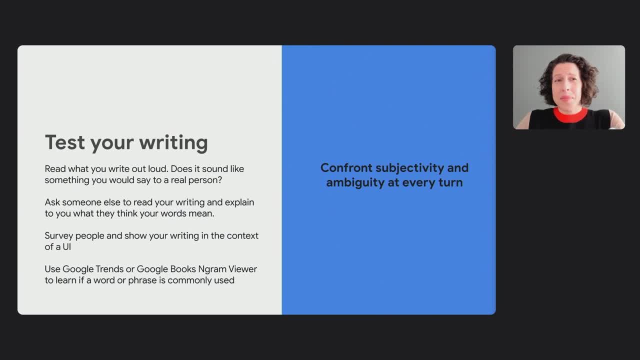 And that's also really important because, like we saw in the doughnut example, you might have your own preferences and habits, but they might not be shared. It reminds me of a mistake I made when I was new to UX. I wrote a bunch of notifications in Google Docs. 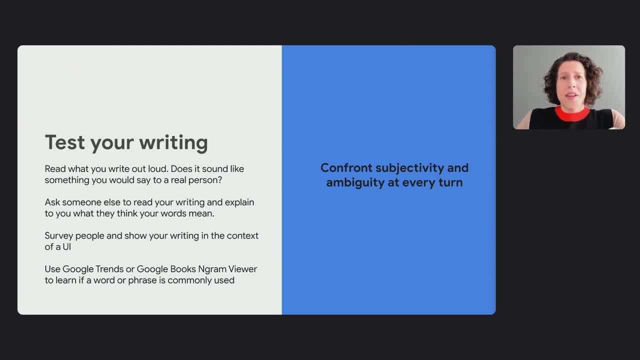 And Google Docs are great for writing, but it's not great for writing UX text. So by writing it without the context of the component and the screen, I just couldn't anticipate what it would be like in the context of an interaction. And in that mistake you can also see a good definition of UX writing and what makes it unique. 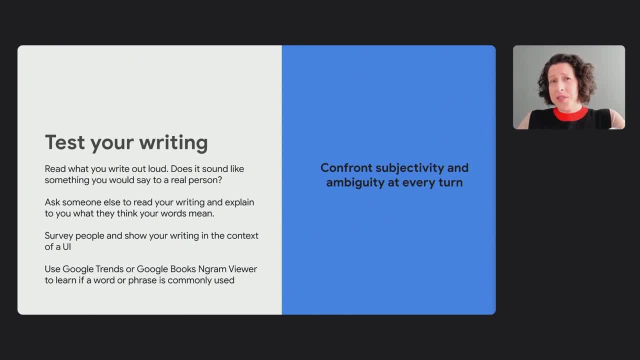 If I were to just stay in the doc, I would have failed. as a UX writer, I had to see it in the context of the screen, the component and everything around it that it relates to to make it right. Some more research methods I want to mention. 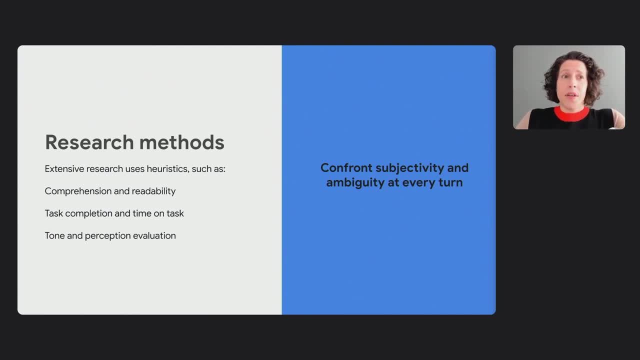 if you do have the means and the time would start to involve more heuristics like comprehension and readability. We're also looking at task completion and time on task And we can also judge perception. So testing is an important step to evaluate if what you've written is clear in the real world. 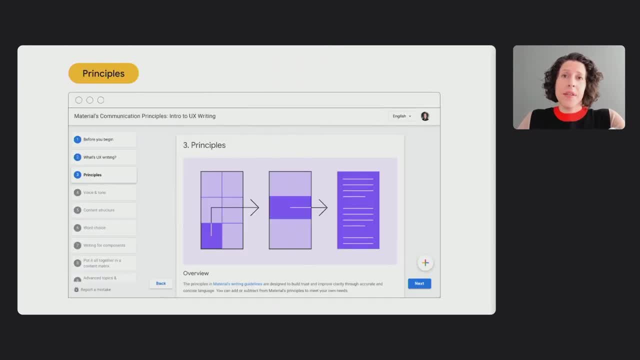 if it has meaning and if it's effective. All right. Step three in the code lab. This is where it gets fun. since we need to bring in some examples to start looking at real words and actions, I'm going to start using an imaginary app called Soil and Water. 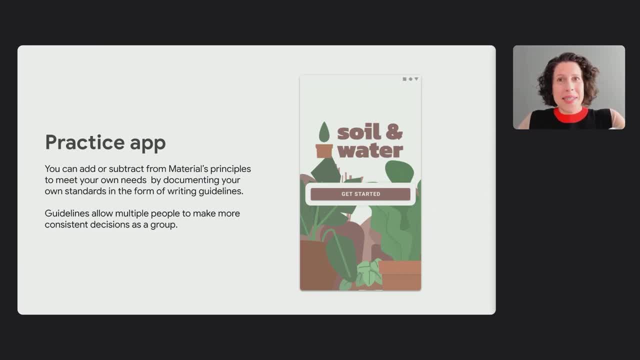 It's an app for garden and plant enthusiasts made by my teammate, Ivy Knight. Ivy also designed another code lab around Materials- Responsive Design for IO- Definitely worth checking out because it covers reflowing text And string length is also really important. 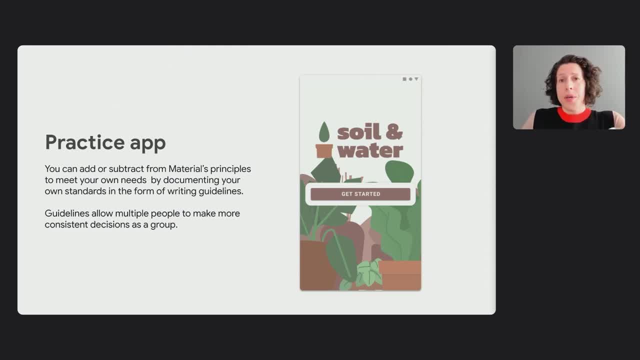 if you think back to the reading pattern in the F shape. So when you adapt your experience for larger screens, the text length is something you can learn about in Ivy's code lab. So we're going to go through some of Materials' communication principles. 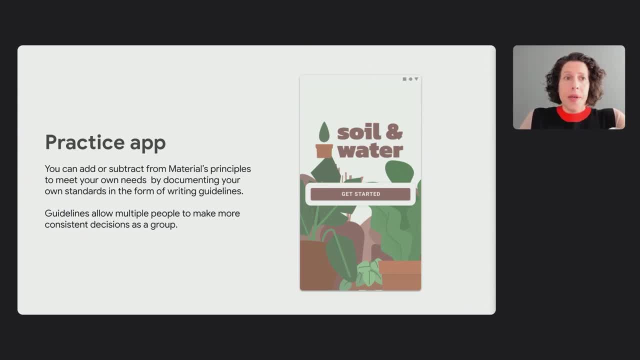 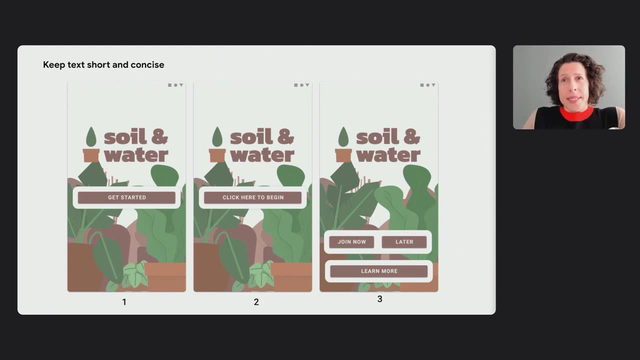 And you can add to these, subtract from them Or write your own. The important part is that having standards in the form of writing guidelines allows multiple people to make consistent decisions as a group. So principles mean that we have a way to create consistent decisions. 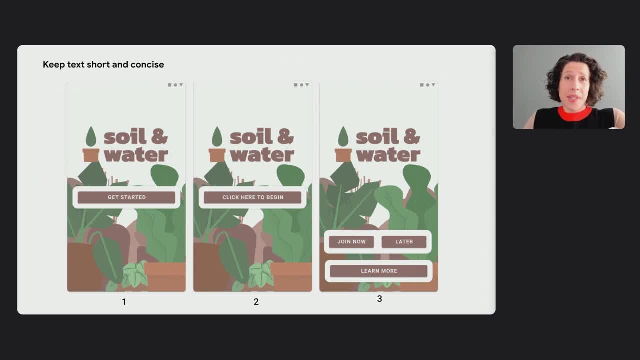 across an organization, across a group of people, And one principle that will take you pretty far is to keep text short and concise. Number one is a good example of that. It just says: get started. This is, This is the entry point for an app experience. 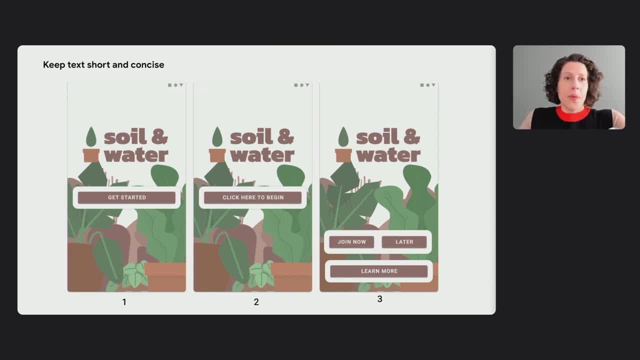 And that's really all you need to say. It's a friendly way to welcome a person. Number two says click here to begin, And it feels a little excessive at that point. Additionally, there's some problems with identifying click here, especially on a mobile device. 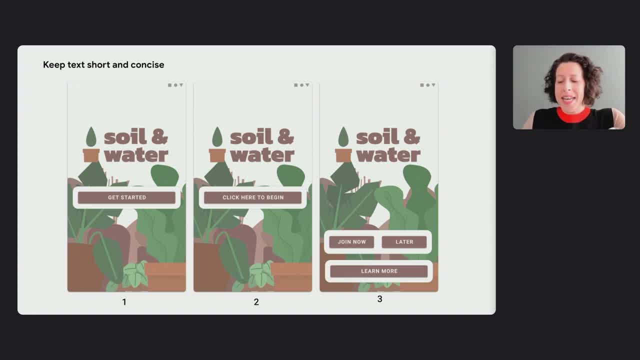 Then the example in the far right is as far from short and concise as we have on the screen in front of us. So join now, later or learn more. Well, a lot of those actions don't even seem necessary, But if you just want to bring someone into your app and make it inviting, 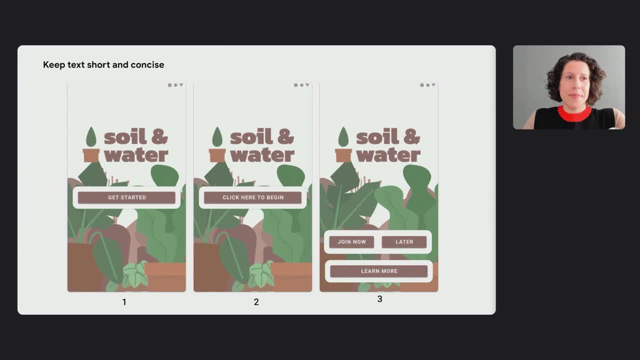 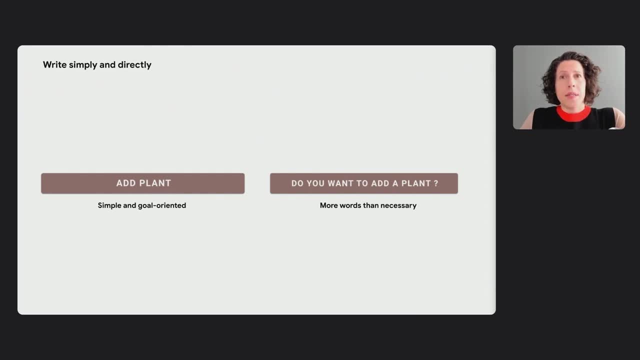 then I would say: keep it short and concise. That's where get started. wins Actions also need to be simple and direct. Space is limited And if you can imagine this is translated into other languages, your button is going to get pretty massive. if you choose the one on the right that says: 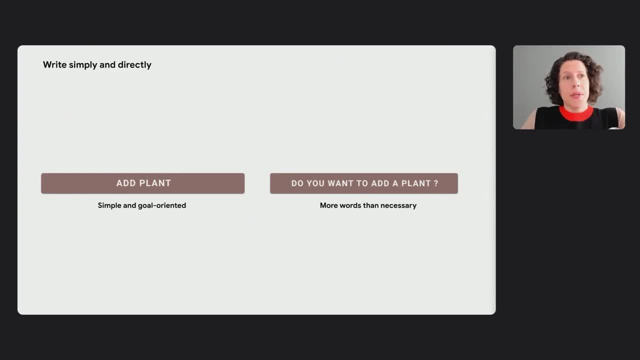 do you want to add a plant. So if you keep things short, if you keep things simple and direct, add plant would actually suffice. And again, this might remind you of the lesson I mentioned earlier about how you don't have to be strict about grammar. 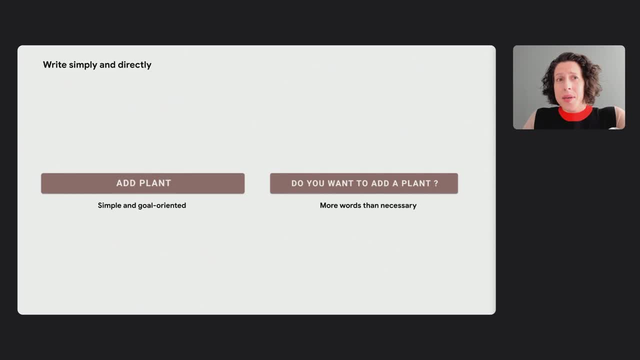 because we are dropping an article there. Add a plant would be a little more proper, But in the context of mobile buttons, keeping it simple and goal-oriented is how I tend to choose my language. Another example from material in the code lab is the idea of save changes. 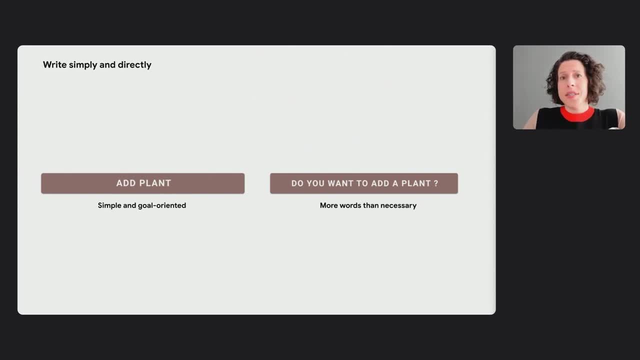 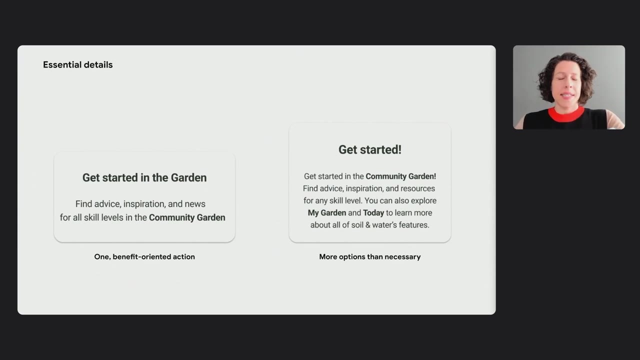 Versus a full string. would you like to save your changes? Both get the job done, but save changes was a lot shorter. This is the principle of just the essential details and not too much at once. So on the left, you can see that in this imaginary dialogue for the garden app. 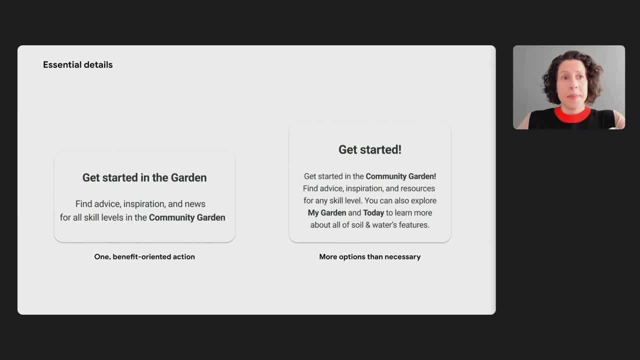 it says: get started in the garden, Find advice, inspiration and news for all skill levels in the community garden. It says that one benefit-oriented action would be all you really need in that context. On the right, you see more options than necessary. 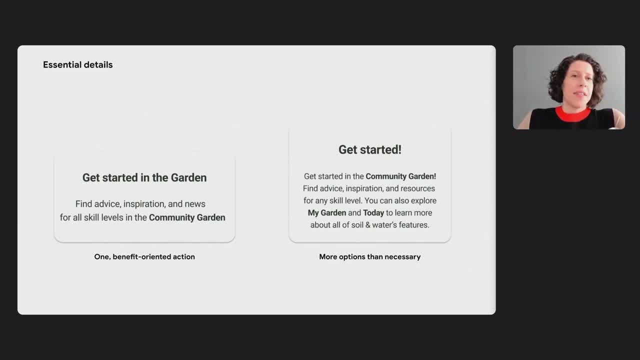 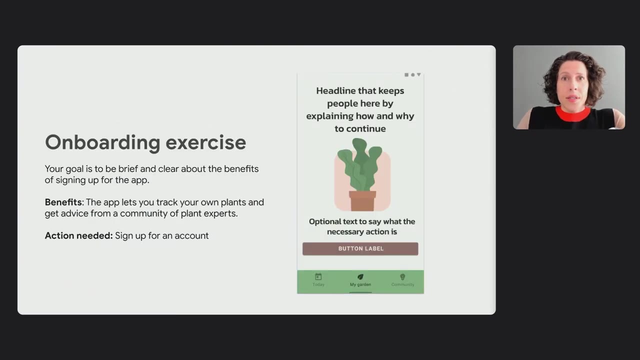 It says: get started, And then there's about four other things you could do from that point forward. The second sentence says you can also explore my garden and today to learn more about all of soil and water's features. That's a lot. So, based on the principles we've covered today, 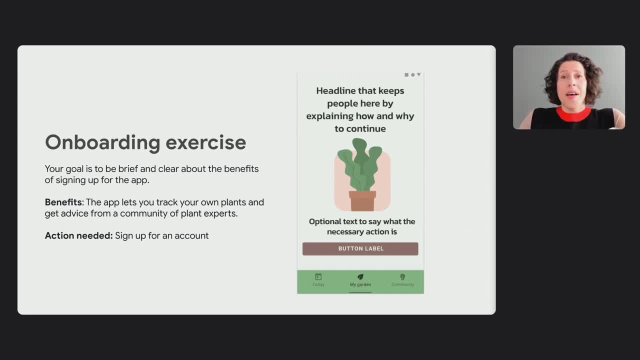 so far, keeping things simple, brief and goal oriented. I'm going to stop here and give you an onboarding exercise. So imagine this is our screen in soil and water. Your goal is to be brief and clear about the benefits that someone would encounter. 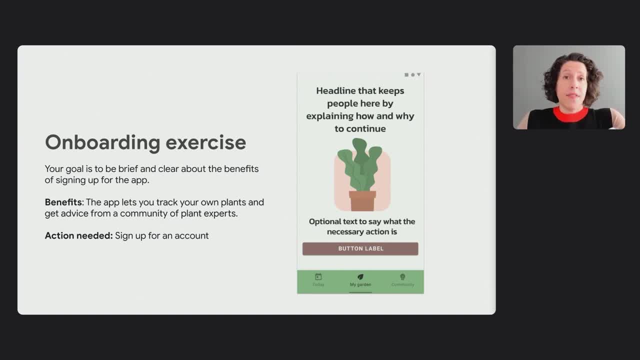 or be motivated by when signing up for the app. The benefits that I'm imagining are that you can track your own plants and you can also get advice from a community of plant experts, And the only action needed is to sign up for the account. 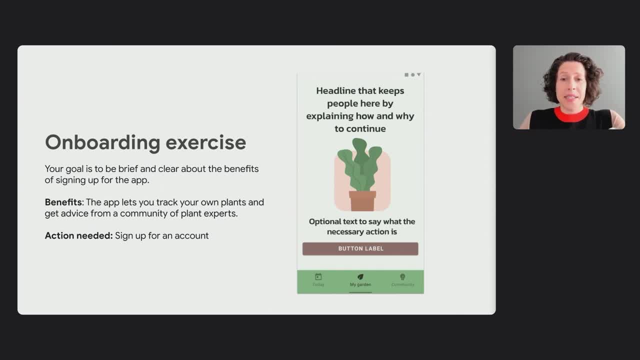 So I'm going to stop talking right now for five minutes, And if you have a piece of paper or a doc open and handy, you can sketch a couple things out. So it's going to be three minutes, two minutes, three minutes. 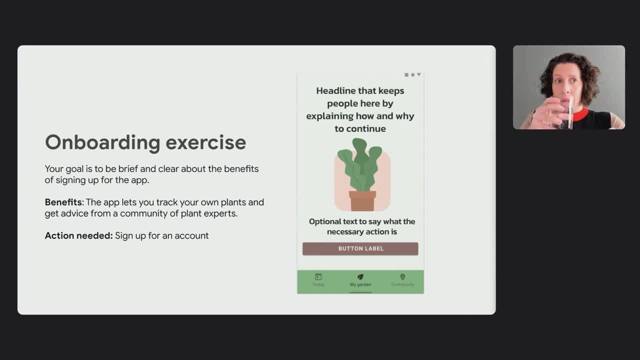 and look at the results And then you can submit those to me. So if you have any questions, any questions, please feel free to ask me And I'll see you in a few days. So if you're interested in learning more about soil and water, 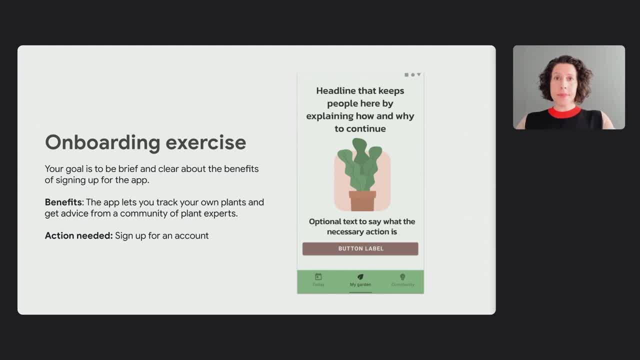 or just hearing a little bit more about soil and water, or if you're interested in learning more about soil and water, I really appreciate it. It's a great time to be able to have a conversation. Thank you, Bye-bye, Bye-bye. 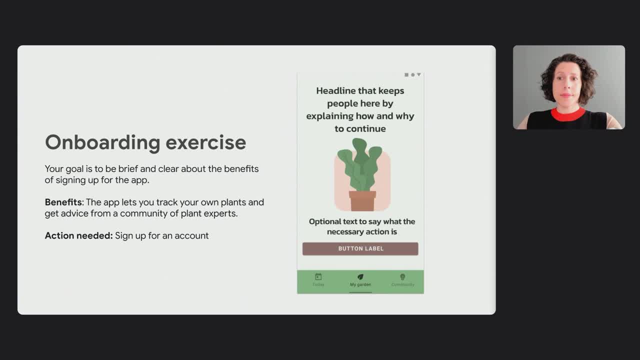 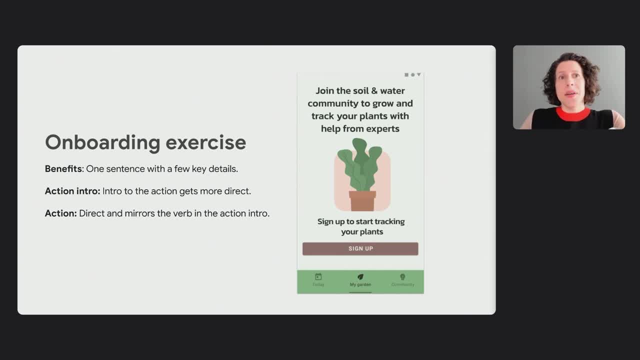 this. I'll just give you my thinking. So, with the benefits I was imagining, I wrote: join the soil and water community to grow and track your plants with help from experts. It's a little bit of a mouthful, but in this context, this is the very first thing you 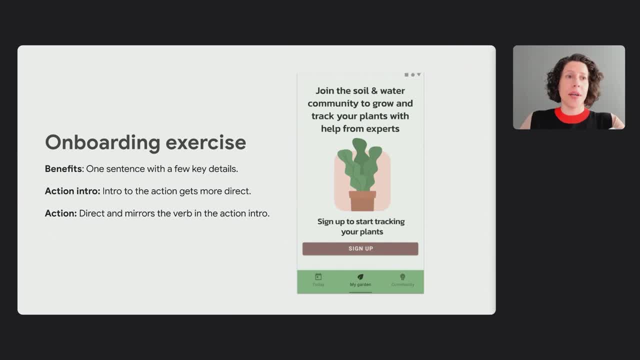 see, so I wanted to make the pitch and the benefits really clear. The line above the button you can see I'm calling action Intro. It's the intro that gets things more direct. It just says: sign up to start tracking your plants, because that's the only action I really 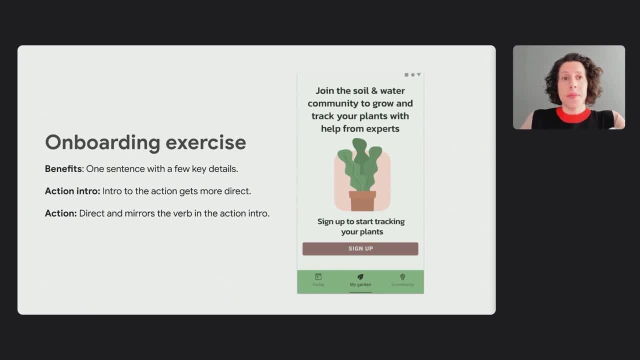 want someone to do in order to advance in the flow, And then the button says sign up. It's direct And the good part is that it mirrors the verb in the action intro. If I said join now in that text, then it wouldn't really make sense to say sign up. 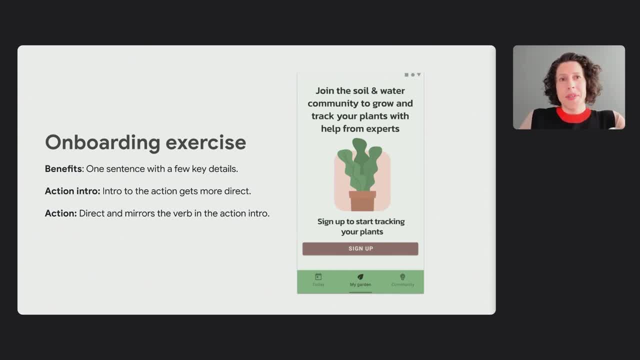 It would raise a lot more questions. So maybe that's it. Maybe think about the choices you made. You can see what I did, And that's also what's fun about writing is that I'm sure ours look different, and I wish I could see them. 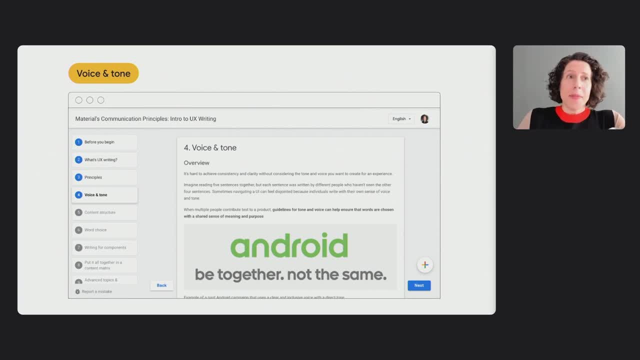 All right. So that was principles and we're on to voice and tone. In the code lab, I used the example from Android: be together, not the same. This is an older example from Android, but I really like it because it's so brief and 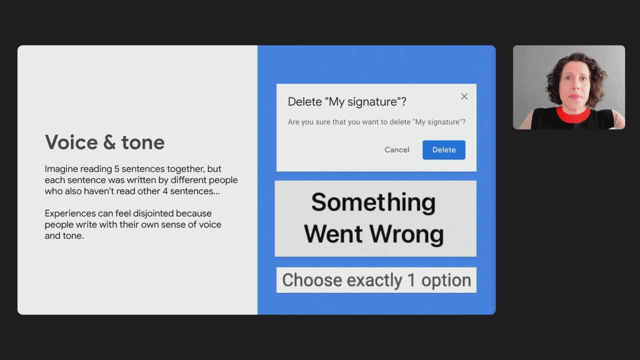 succinct, but it's also inclusive and clear. Okay, When multiple people contribute text to a product, it really helps to have guidelines for tone and voice. It ensures that the words that are chosen, they have a shared sense of meaning and purpose. 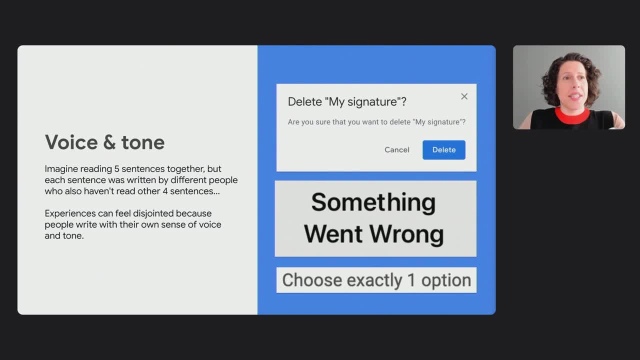 So imagine reading five sentences together, but each sentence was written by different people and they haven't read the sentences that the other four people have written. So you can imagine that would create a pretty disjointed experience. People write with their own sense of voice and tone. 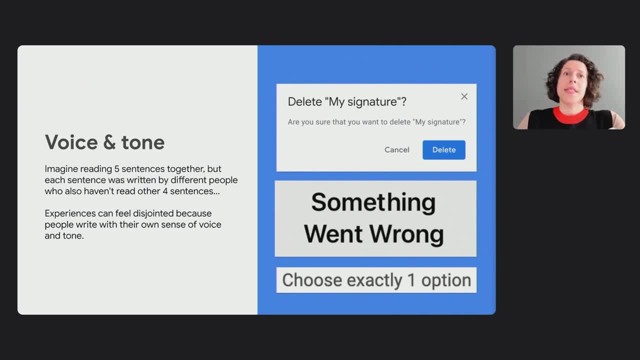 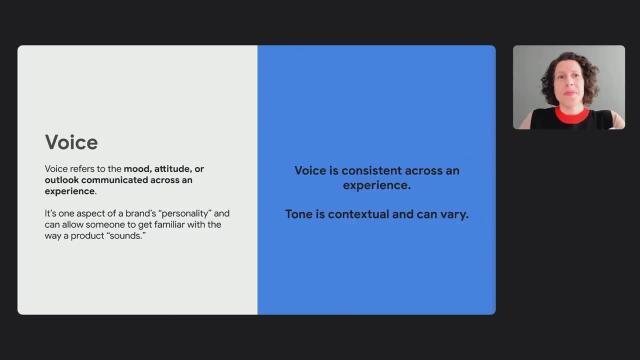 It would be as though these examples on the right side of the slide here were all from the same app experience. That would be a little weird. So what is voice? Voice is the thing that you try to keep consistent across an experience. The tone is contextual and can vary. 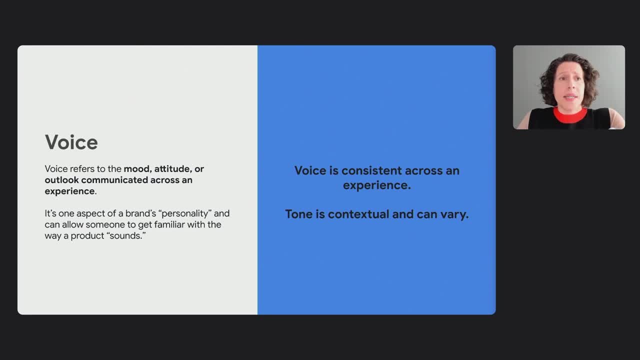 It refers to the mood or attitude that's communicated in an experience. It's an aspect of a brand, personality, It's the thing that might lead you to say, oh, that sounds weird, That sounds like something Google would write. And, ultimately, what an individual considers a good example of voice, like helpful, accessible. 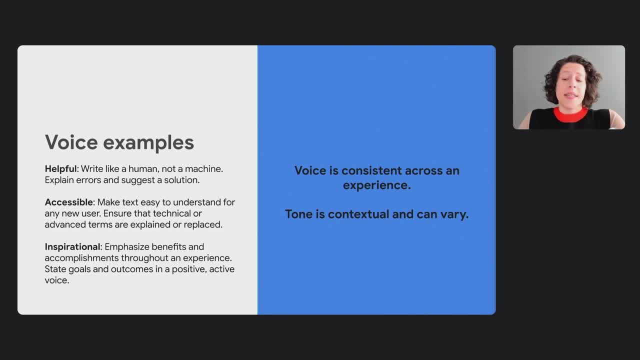 or inspirational. it will also vary, And that's also where sensitivity, cultural context comes in as well. So here are just a few examples. If I said I wanted my voice to be helpful, I would describe it and create some examples around the idea of writing like a human, not a machine. 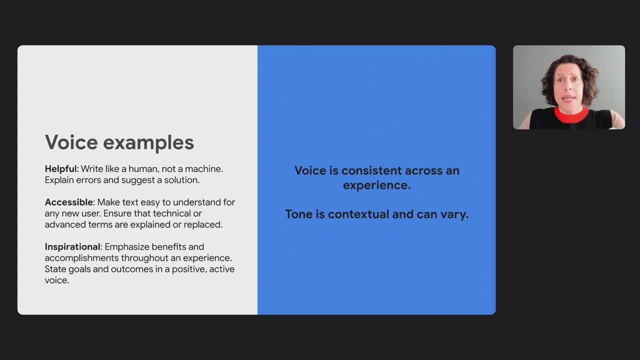 I would describe it and create some examples around the idea of writing like a human, not a machine. I would say: any time there's an error, I need to suggest a solution. That would be helpful. Let's jump to accessible, So that would be a way of making text easy to understand. 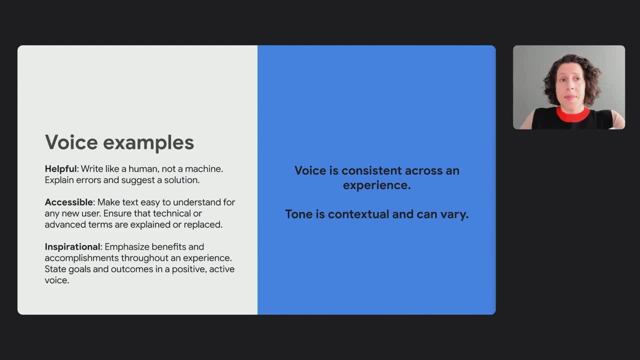 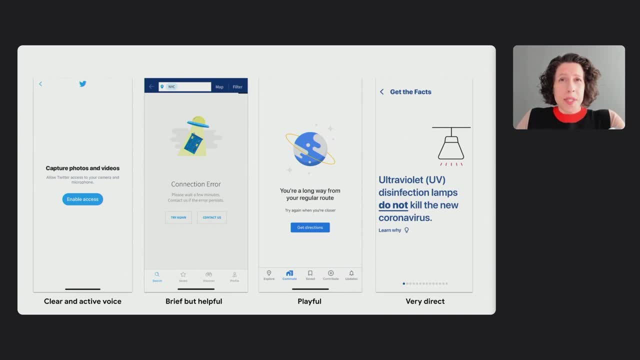 So no advanced technical terms, And any time I do need them, I would explain or replace them: Voice principles, guide, word choice, and they really do benefit from examples that illustrate it in action. Otherwise, it would be a little too abstract to get multiple people to make similar decisions. 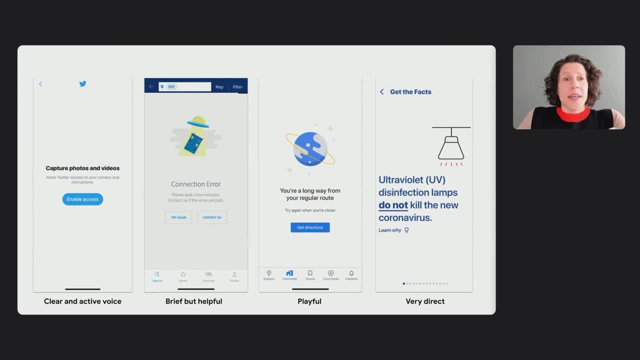 So you might remember these screens from earlier And they show a little bit of. they show a few different voices. The one on the left is active, It's clear, It's very direct. This one that I'm calling, brief but helpful. it starts with connection error. 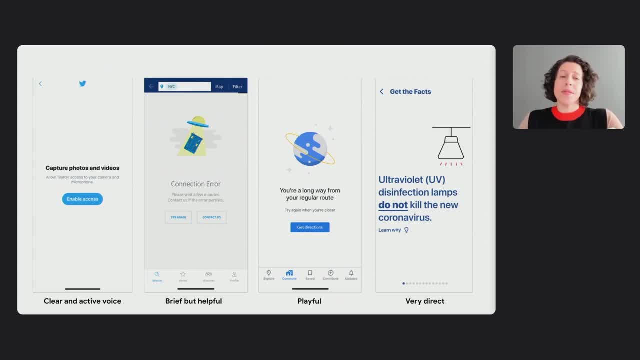 So you get the message very easily. But then the next line begins with a please. So they kind of want to have it both ways. All right, Bye, Bye ways. The next one is playful. It says you're a long way from your regular route. Try again. 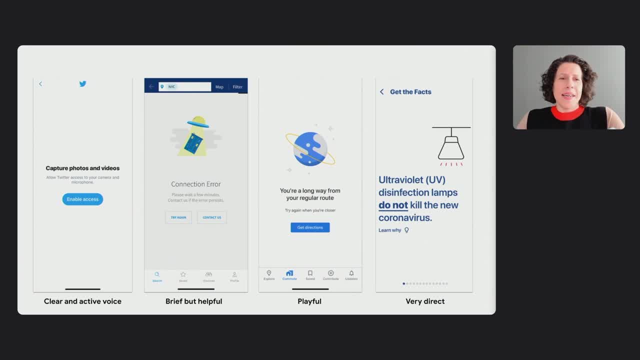 when you're closer. So that's in Google Maps And I maybe tried to navigate home, but I was way too far away And that's fun. I think it feels lower stakes And they can afford to be playful in that space. Then on the far right is the COVID app And it's very direct Ultraviolet. 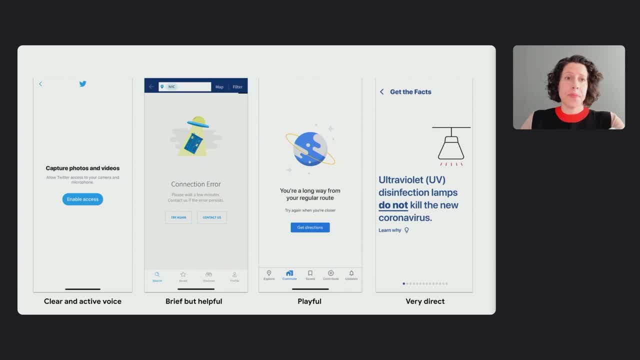 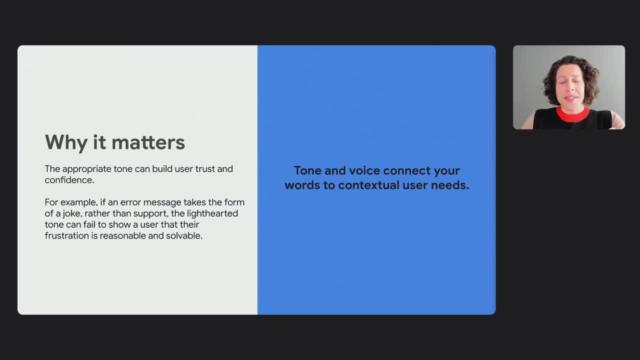 disinfection lamps do not kill the new coronavirus. Why it matters is that the appropriate tone can build user trust and confidence. So imagine if the ultraviolet lamp was ironic or used a joke. That would just take a scenario that shouldn't be lighthearted And it would 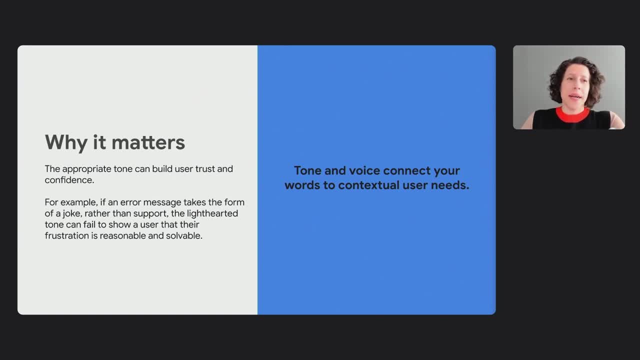 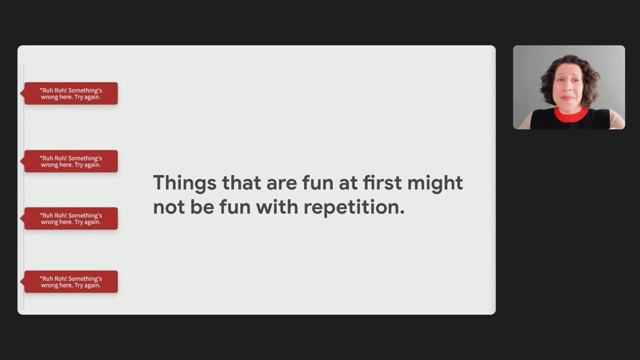 fail to show some empathy. And then, when it comes to errors, having the right tone helps. It helps the user feel that their frustration is reasonable and solvable. And one more example is to say that things that are fun at first might not be fun with repetition. Another reason: 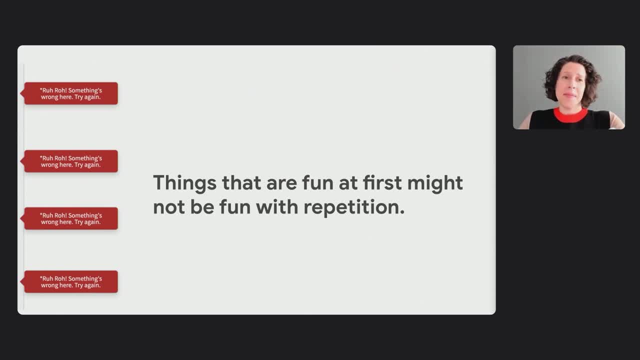 why you need to start tracking content decisions and documenting them. So something that seems like it would be delightful once falls into this kind of problem of habituation. Error states are usually a key example of that. So you can use an example of where tone mapping can help inform a shift in tone that takes. 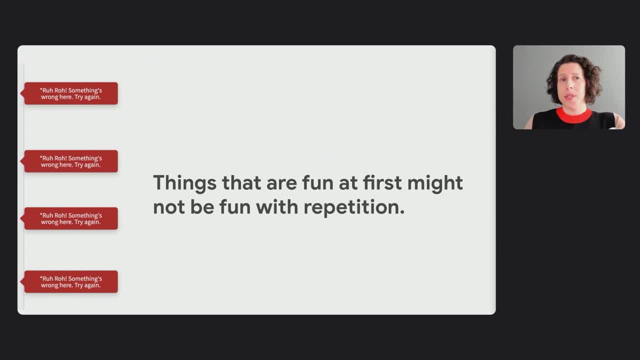 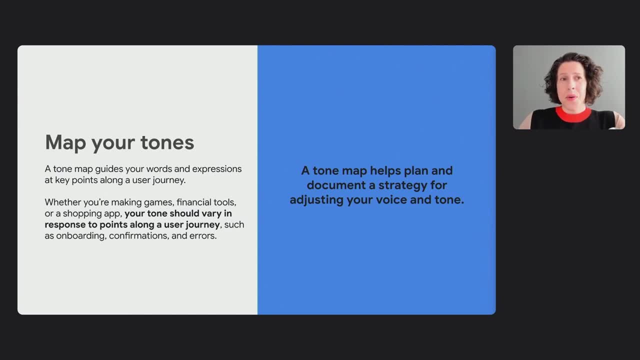 something casual and conversational into a more supportive and appropriate space. So, mapping your tones: We're going to do a tone map And that's something that will help you plan and document a strategy for adjusting your voice and tone across an experience. The tone map guides your words and expressions and whether you're making games, financial. 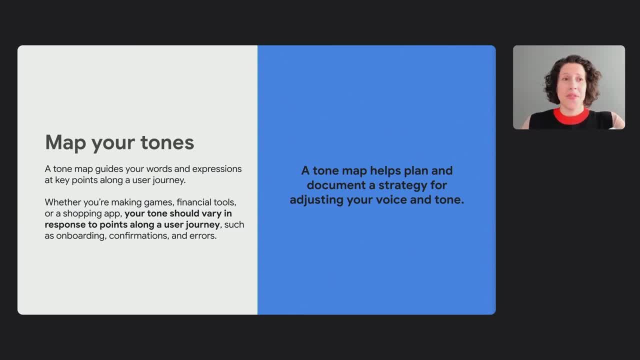 tools or shopping app. it might help if you're making a face to face conversation Where app, as I imagine, everyone is doing their own thing. your tone should vary in response to points along a user journey. So, whether it's onboarding, confirmations and errors, 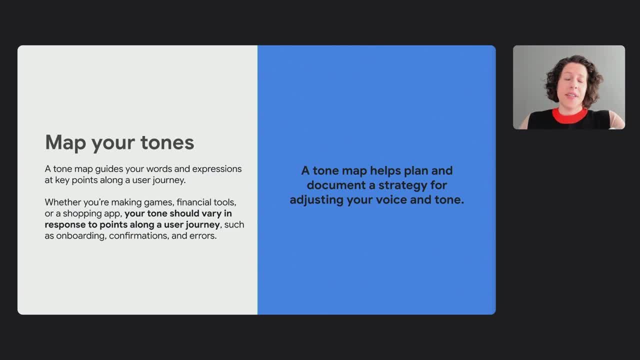 if you're the game app, you don't always want to be funny, And if you're a financial app, you still have a range in between scenarios that are very serious and some where you just want to be easy to understand. So we'll walk through this one together. It's the tone map. 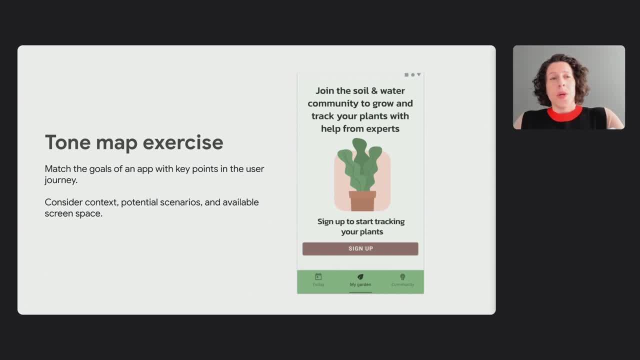 exercise, And so we want to imagine the goals that take the user goals of an app and match them with key points in the user journey, And you'll consider the context, the potential scenarios and the available screen space when you make these choices. So the first step: 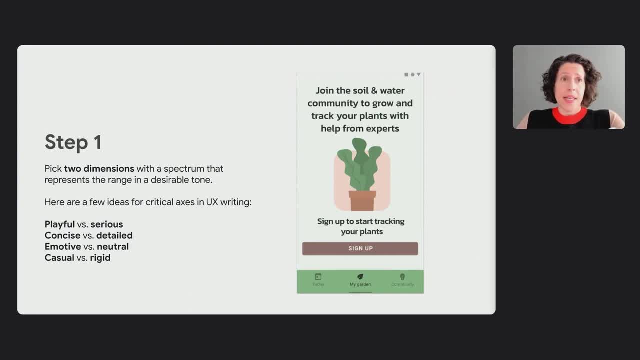 is to take two dimensions, pick two, anything on a spectrum that represents the range in a desirable tone. A few common axes In UX writing that are critical would be playful versus serious, Concise versus detailed, Or it could be emotive versus neutral, It could be more casual or rigid. So consider: 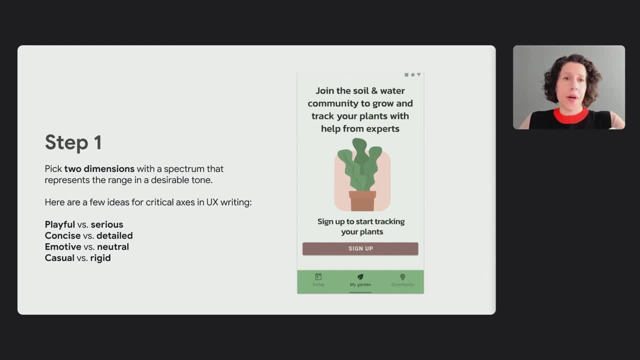 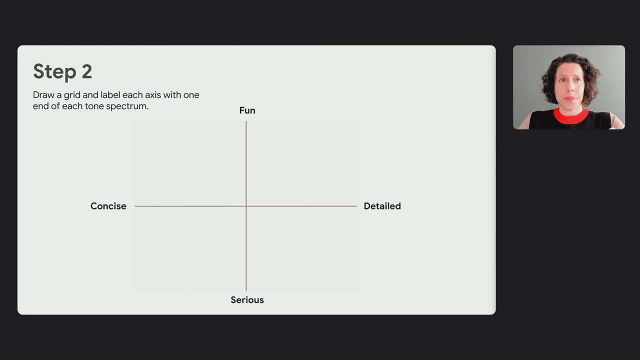 for a second. what dimensions might matter to something you're working on, or what makes sense to soil and water? In step two, take your piece of paper And draw a grid and label each axis with one end of the tone spectrum that you selected. 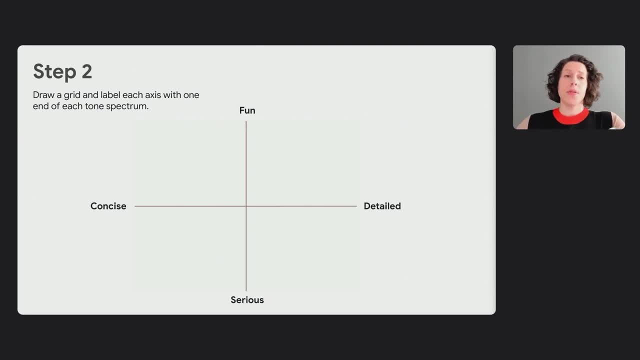 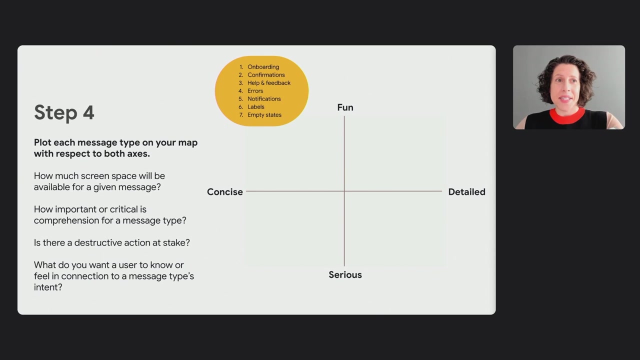 Another way people often do this is with chronology. They would map the user journey instead. What we're going to do in step three, then, is I've listed the message types, or common language patterns, And I'm going to give everyone four minutes to think this through. How much screen space? 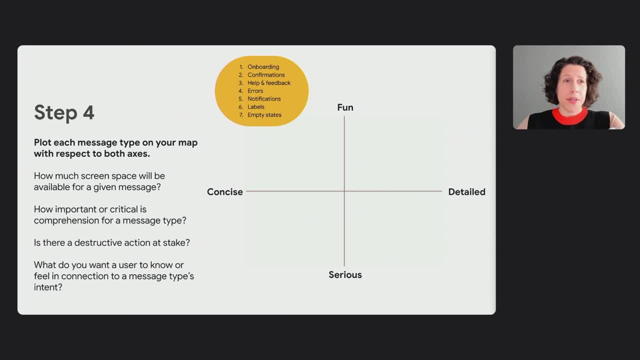 will you need for a given message? How important or critical is comprehension for this message type? Would there be a destructive action at stake? Would there be a negative action at stake Or do you want a user to know the message type? So I'm going to give you four minutes. 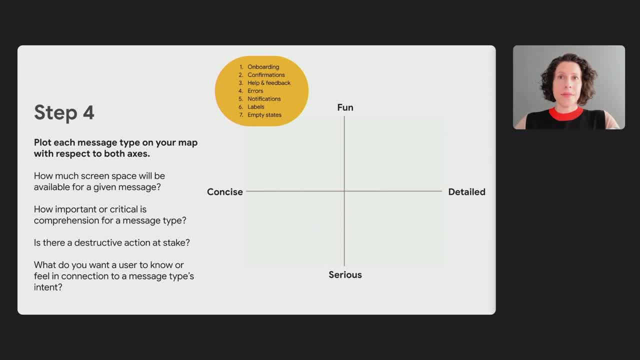 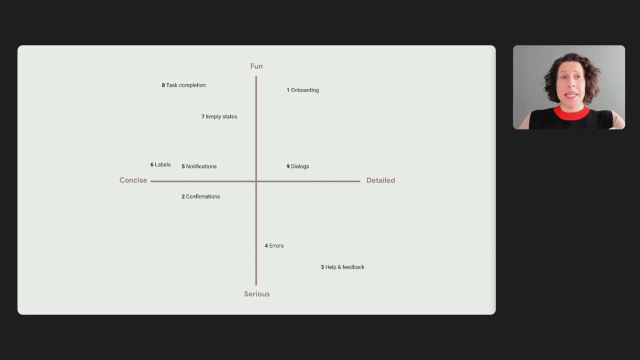 I'm going to share my screen with you right now: One, two, three, four, five, six, seven, eight, nine, 10.. Thank you, All right, let's take one more minute. All right, here's what mine looks like. 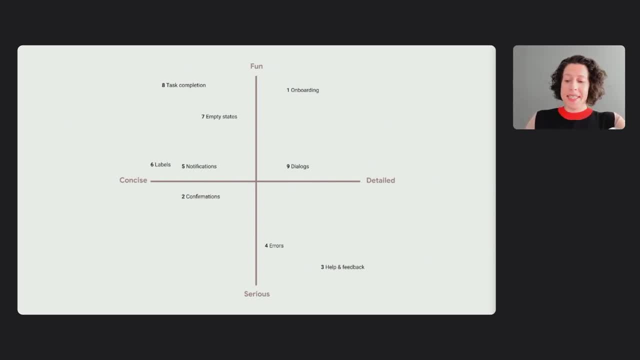 I charted fun to serious and concise to detailed. You can see onboarding is pretty high up on the fun meter. It doesn't have to be fun but it just doesn't require so much seriousness in tone. On the other end of the spectrum- at serious, detailed is help and feedback and errors. 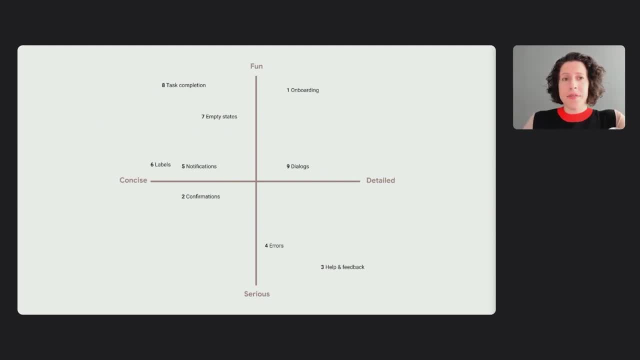 Those are situations where you need to give the right information, and it's better off if it's not a joke In the case- if we look at the top left task completion- I slotted that. I charted it as something that you can probably have a little fun with in the case of soil and water. 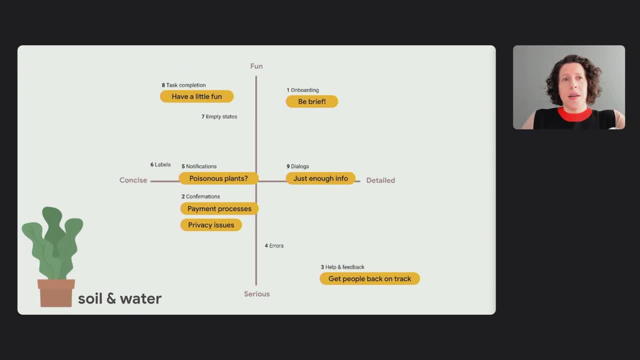 But if you look down to notifications, I started thinking through the possibilities for soil and water. Well, if I'm adding a poisonous plant to my garden, I would definitely want to be notified, and something that felt at first like a hobby app actually became like a life and death scenario really quickly. 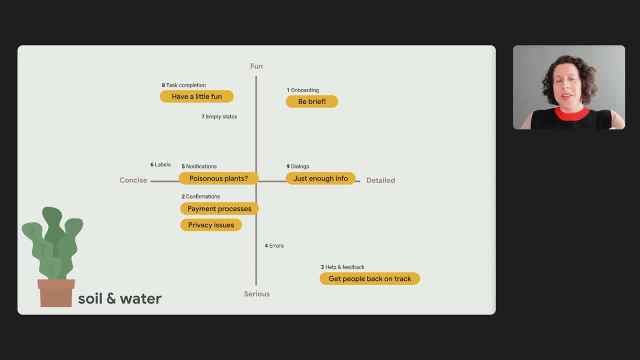 So you know it doesn't. I didn't want to chart everything by default into the fun space just because we're talking about gardening, which is a leisure activity, And that's the whole point of a tone map, which is that I can think it through. 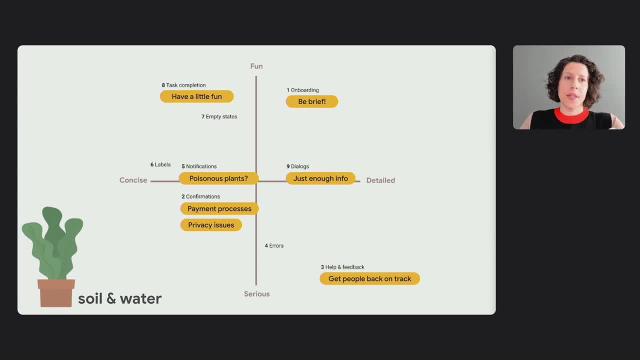 and look at how each type of message relates to each other. Another important one is confirmations. So I'm imagining soil and water. So I'm imagining soil and water has a shopping page and in that case, payment processes and privacy issues are imperative. that they're concise. 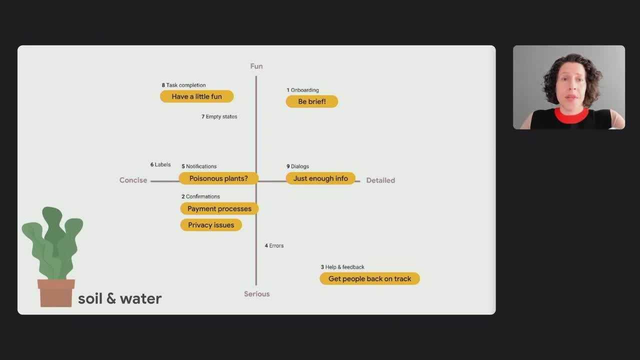 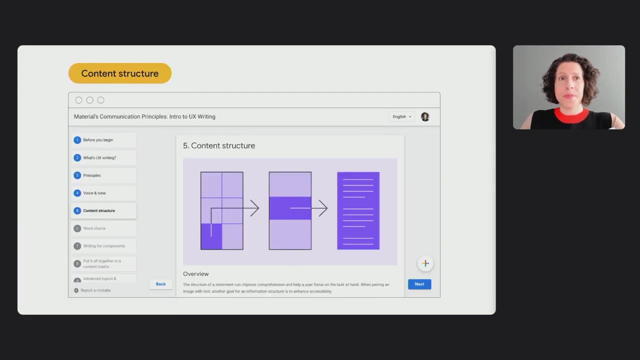 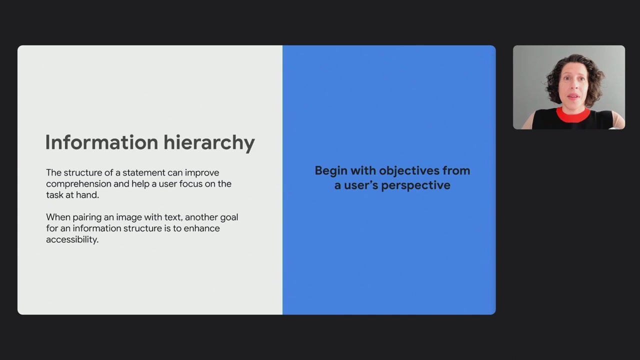 serious and handled with a lot of care. I'll leave this up for just one more minute so you can compare it to where you put your message types. All right. moving on in the code lab, we get to content structure. What does that even mean? 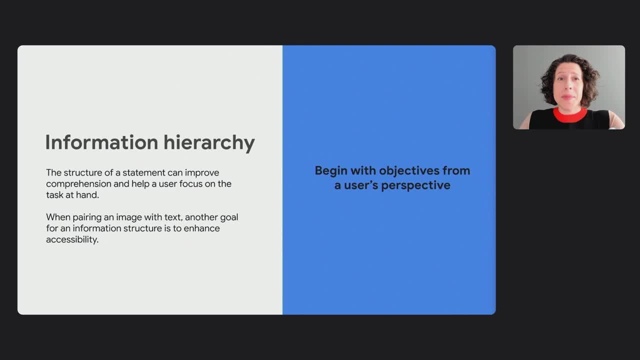 It means information hierarchy. Sometimes people say information architecture In the case of materials, communication principles. it's the idea that we want to put the user's objectives in the front of any statement and put that perspective above all others. So when we say information hierarchy- 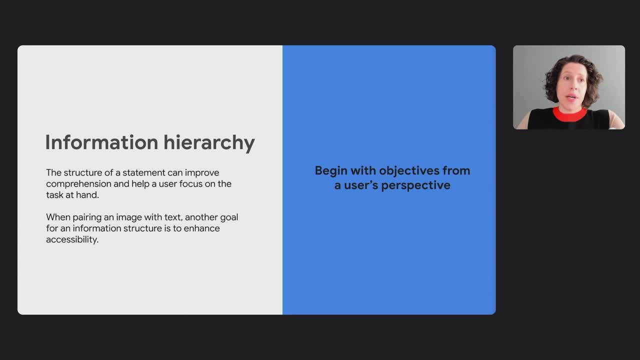 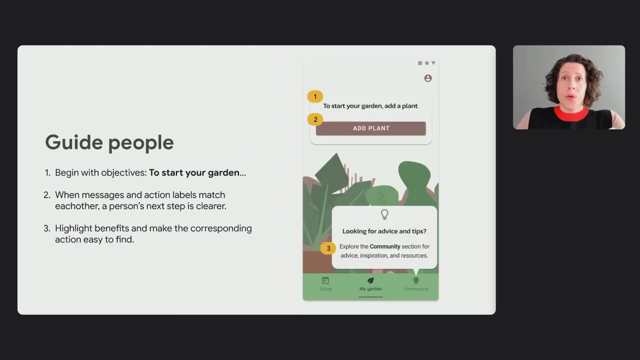 we're thinking about how the structure of a statement can improve comprehension And it really just drives home this idea that it's goal oriented And that another key aspect is enhancing accessibility. So content structure is there to guide people If you begin with an objective like start your garden. 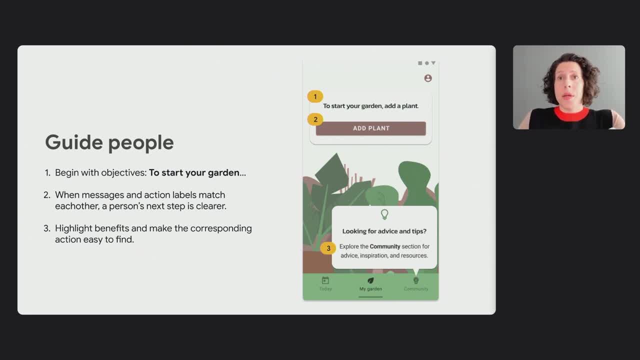 that will help begin with the benefit. So it puts the task oriented pattern in the front of the statement. Experiments can be redefined on this- And it introduces a strongly looking framework for a task rather than adding a plant because I might say, well, why do I want to add a plant again? 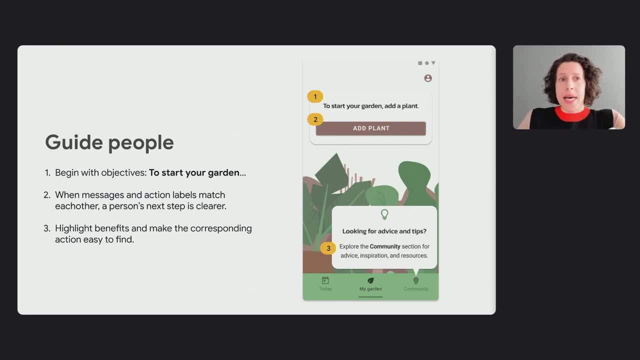 So the next thing is to add the plant In that button. we see that the message and the action labels match each other, and that makes the next step a lot clearer, All right. finally, in that bottom diagonal, we're able to highlight Facebook benefits. 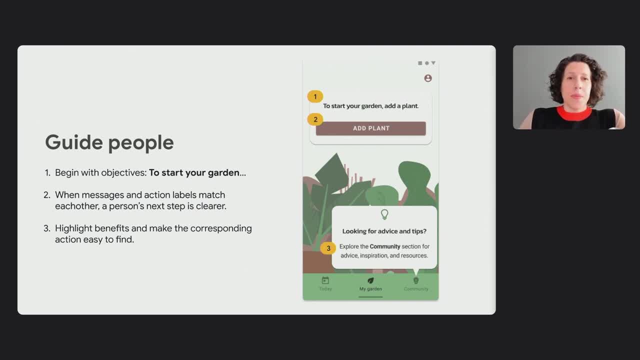 So the the word community is bolded, and that's because we want people to see the connection between the navigation bar destination called community and the thing we're talking about in the dialogue. Revealing information contextually and as needed is an approach often referred to. 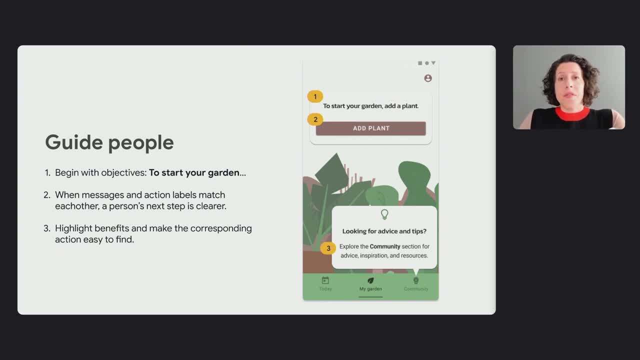 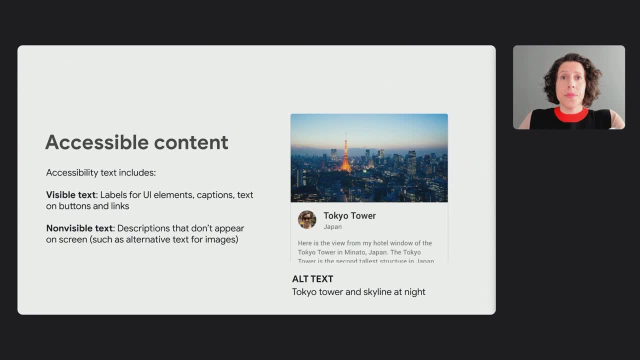 as progressive disclosure, but I think of it generally under the whole goal and the bucket of guiding people through a hierarchy of information. Effective writing extends to the considerations of image and text pairing for users with low vision and anyone using a screen reader, When both visible and non-visible text is descriptive and meaningful. 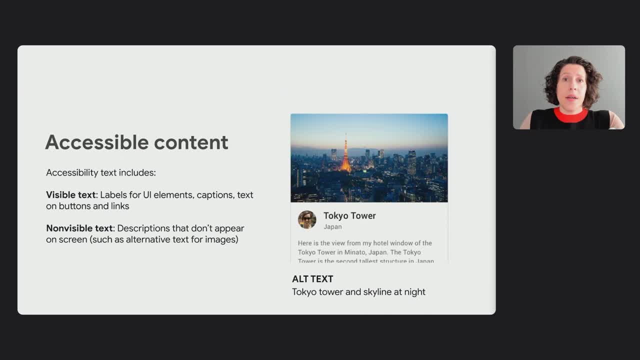 it helps users navigate headings or links on the screen. A screen reader can help you test accessibility text and identify places where you can add it. My teammates worked on materials accessibility writing section, which I highly recommend. It includes guidance for pairing images and captions so that it 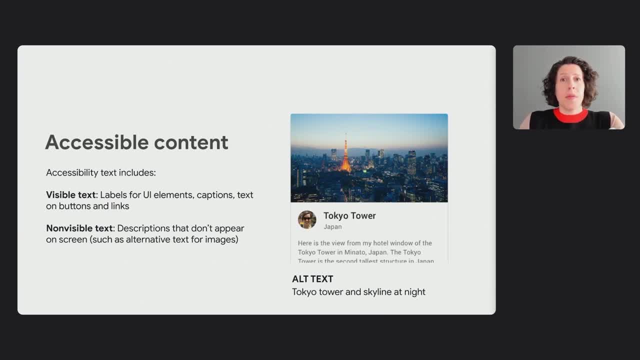 is easy to understand the content design. The important part here is to think about also the text that you don't see. So alt text for this image of Tokyo tower might read: Tokyo tower and skyline at night. And if you want to learn more about writing alt text, I definitely recommend the material article. 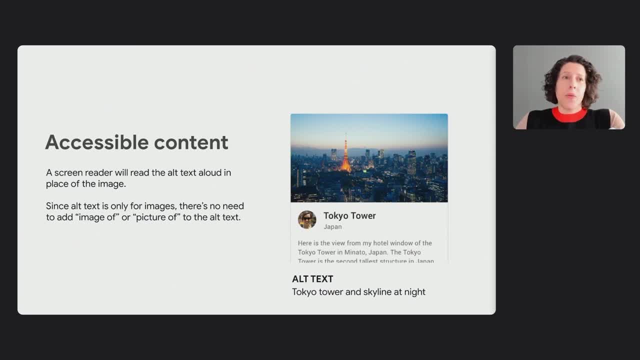 It will tell you some of the more considerations about what a screen reader or what a screen reader will say out loud in place of the image, Because it's important to consider a few key dynamics of how the screen reader articulates text. For example, number one: you don't need to say 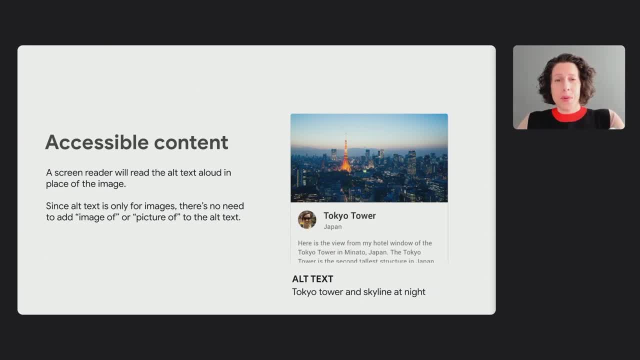 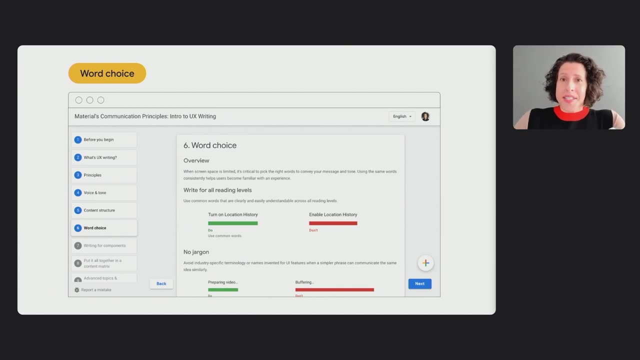 image of or picture of. Often times when people are writing alt text, at first they might have written picture of Tokyo tower and skyline at night, But actually that's already known. So those are some basics on copywriting. I'm going to jump straight into word choice now. 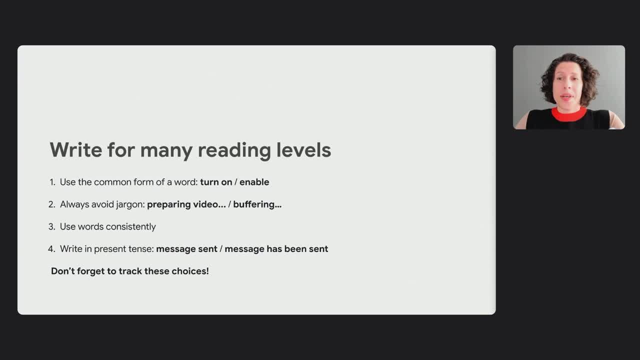 There's a lot of things we can talk about word choice- I won't go into grammar too much- But mostly the important principles, which are that you want to write for many reading levels. I try to use the common forms of words like turn on or enable. Turn on instead of enable. 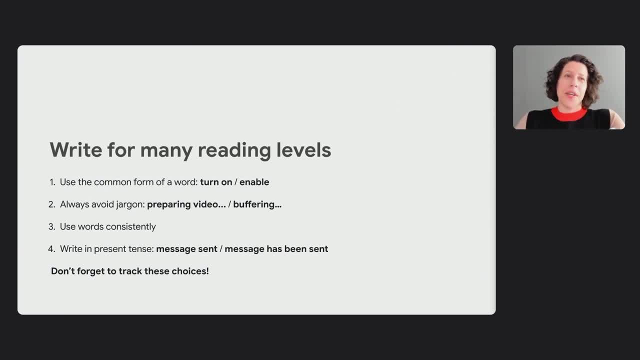 And one of the most important things to remember is to avoid jargon. So something like preparing video is a much easier way to say buffering. So we also try to use words consistently And to write in present tense. Present tense is message sent. Message has been sent means the same thing, But it does it with a few more words. 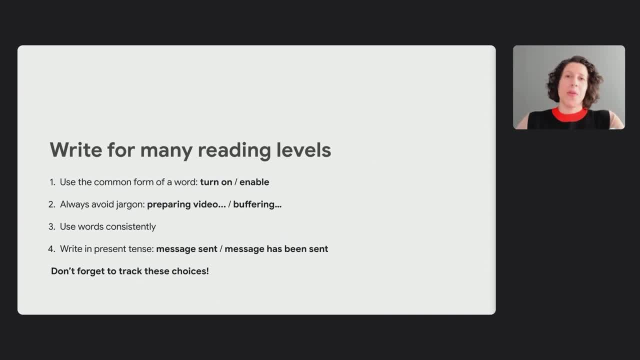 And once you start making choices like these, don't forget to start tracking them in a word list, Google and material design communication guidelines. we usually say used to say write for all reading levels, But to be more specific, what we're really trying to do is write for equity and inclusion. 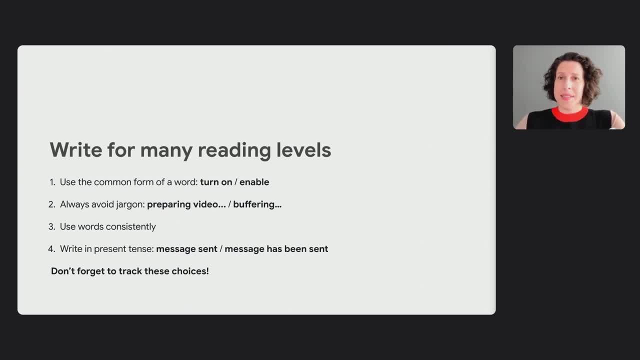 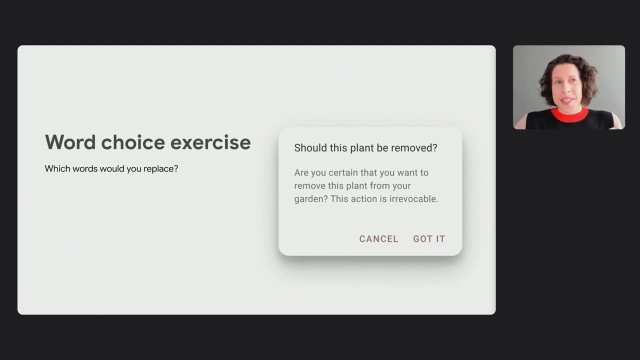 It's a little hard for me to imagine what all reading levels means, So just thinking about your user and what kind of word choices they use is always a good place to begin. Here's a little word choice exercise. I'm going to give you one minute to read through this dialogue. 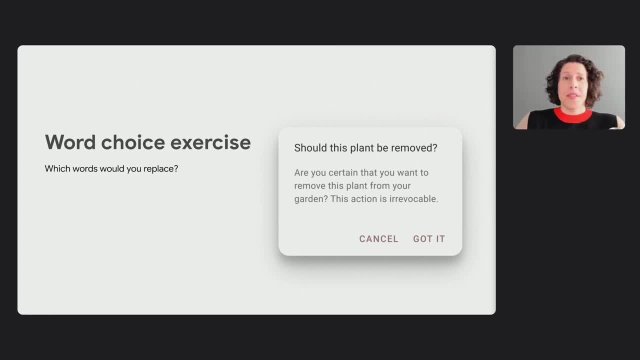 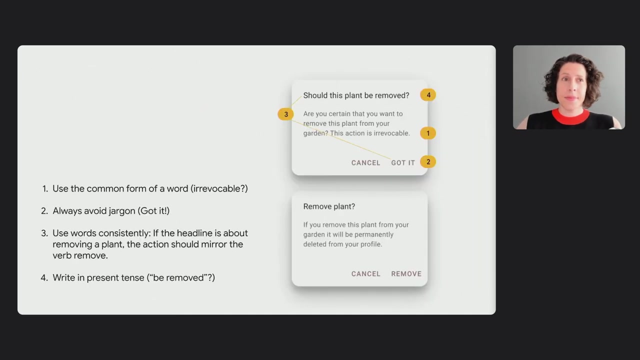 And think about which words you might replace Should this plant be removed. Are you certain that you want to remove this plant from your garden? This action is irrevocable. Your options are: cancel and got it. So I did a little rewrite below: 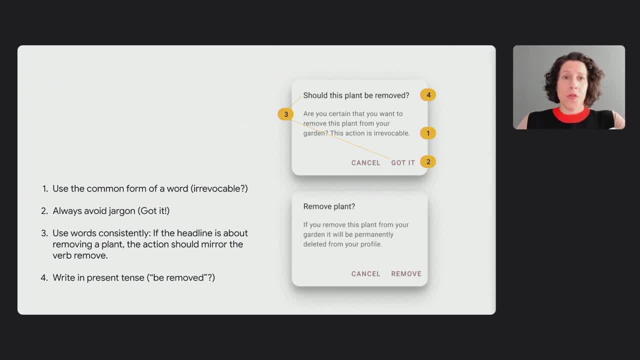 Mine was remove plant. If you remove this plant from your garden, it will be permanently deleted from your profile. The options are cancel and remove. So first off, I hope you spotted the word irrevocable- That's a pretty fancy way of saying the same thing, which is permanently deleted. 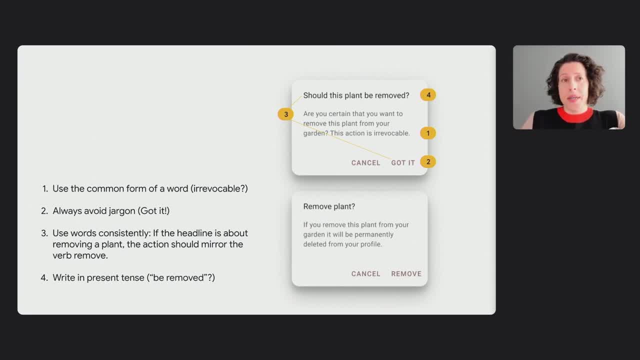 Sometimes people will really get interested in the technical nuances of where the documents are. So sometimes people will get interested in the technical nuances of where the documents are. So sometimes people will get interested in the technical nuances of where the documents are. the deletion happened. But ultimately, if you want to offer all the details of the data, 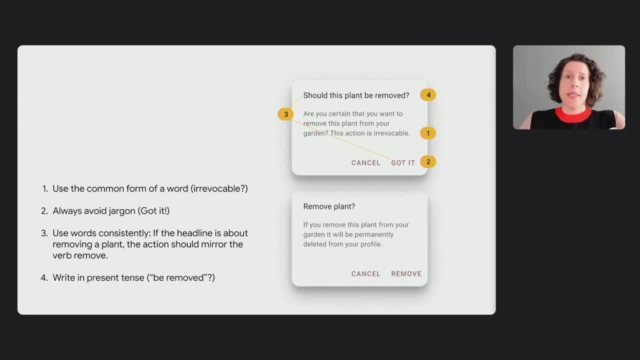 storage. you can add a learn more link or put that in another space in the app. So another thing that I felt was jargony was the word got it. You see that around Google a lot, But when we're talking about destructive actions where something is at stake, a permanent- 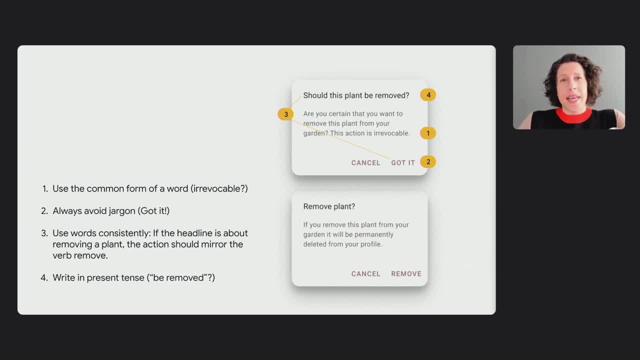 change. I felt like got it was a little too insidery. If you haven't used a lot of hobby apps before, maybe you haven't really confirmed important actions with a phrase like that. So remove felt like it was more aligned with the headline Remove plant, Yes, remove. 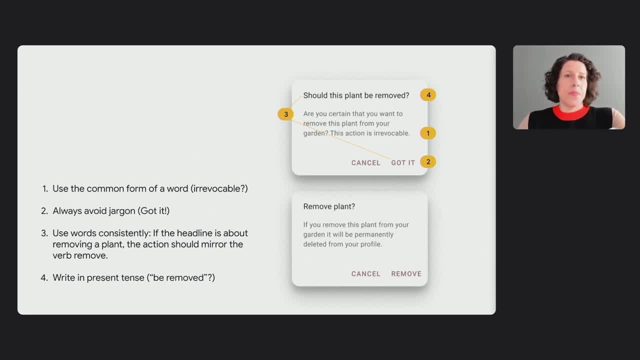 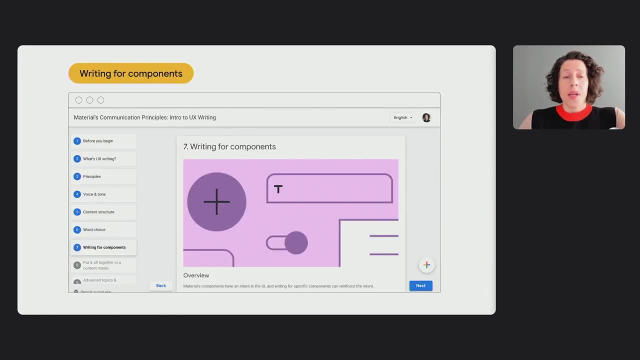 And another smaller note is that the original headline said: should this plant be removed? So that's a saying: to be removed. But remove plant is a lot more direct. It's the principle of present tense. So in the code lab we get to writing for components. It walks through some of the materials: components. 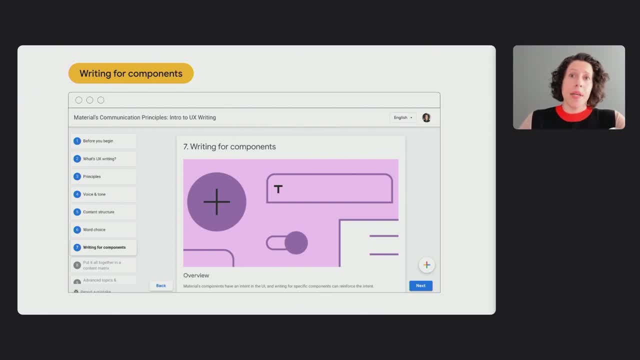 that you've actually already seen in use in a lot of the example app Materials. components have an intent in the UI And writing for specific components can really reinforce that intent. If you go to that section of the code lab or materialio, you'll see writing guidance. 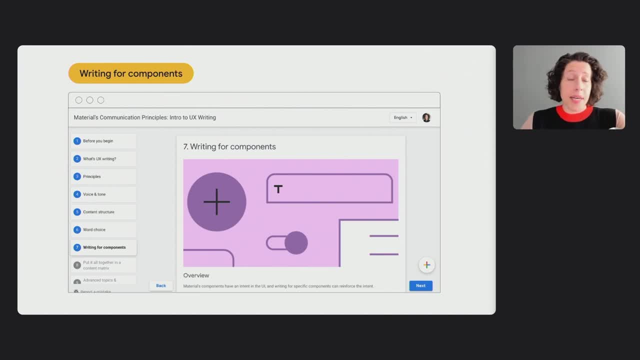 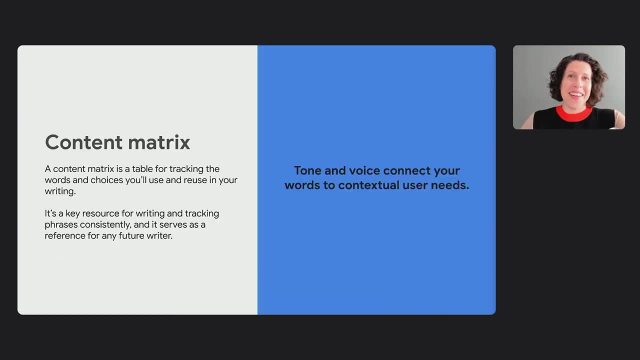 for dialogues: cards, chips, snack bars and text buttons. All right, You've almost made it, So now we're at the stage where you put it all together. That's a content matrix, Which is actually a fancy name for a spreadsheet. And yes, I broke my rule about. 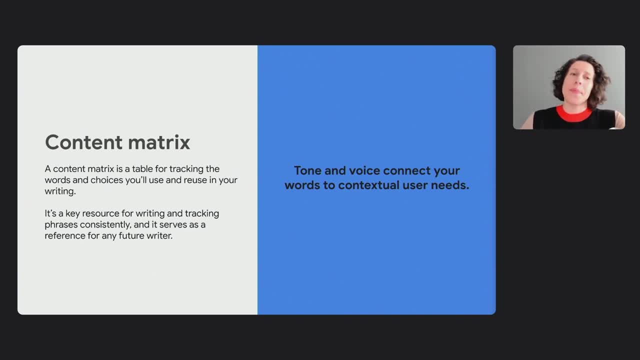 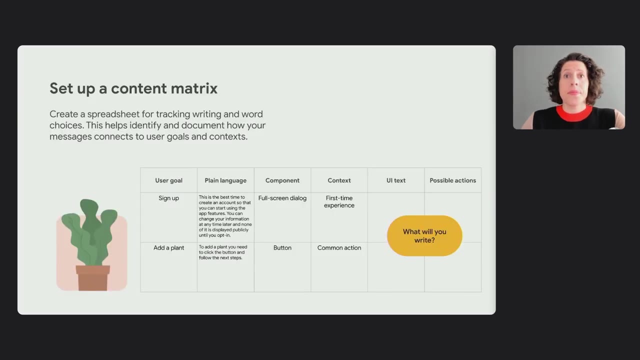 word choice Guidance for no jargon, But here we go. The content matrix is what we call a table for tracking the words and choices that you use and reuse in your writing. It's a key resource for writing And tracking stuff- for yourself, But also any future writer. How to set up a content. 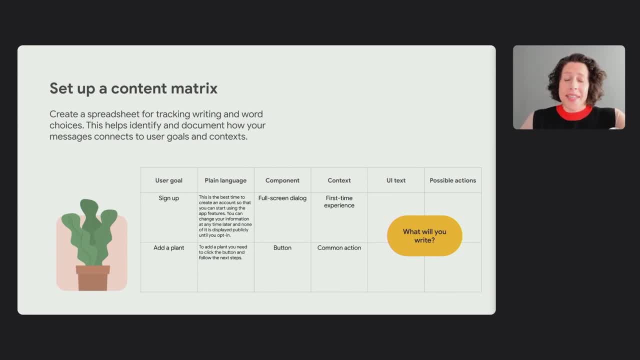 matrix. So you'll create a spreadsheet. Like I said, it's really just a table or a spreadsheet And what you're trying to do is track the words and the decisions that you're making and how they correspond to the points in the user journey. So a table like this would 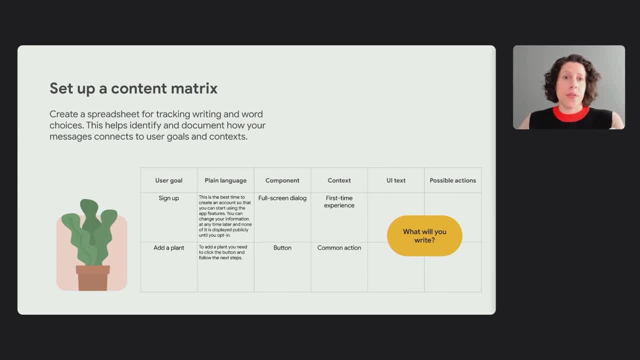 help you identify and document how your messages connect to each element that you want to be thinking about In terms of meeting that goal-oriented text. So you might put in your matrix things that reflect also the tone and voice, principles And you can see I've also 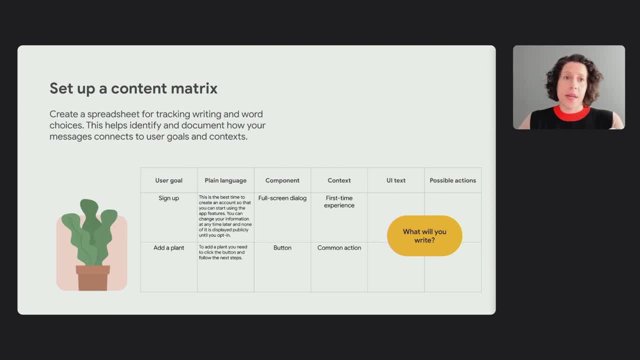 listed component types. So if something is a full screen dialogue, that's definitely something to think about As opposed to a button. Those have very different character lengths. And finally, I would also suggest you put a word list in your content matrix So you can see. 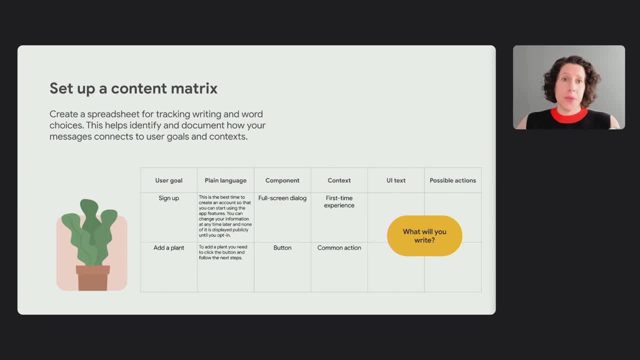 So you list the words and terms that are going into the UI text, and any way that you describe your features or actions or goals are things you want to keep repeating rather than reinventing new ways to say them down the line. You can also list some of the words that should be avoided as synonyms or unhelpful phrases. 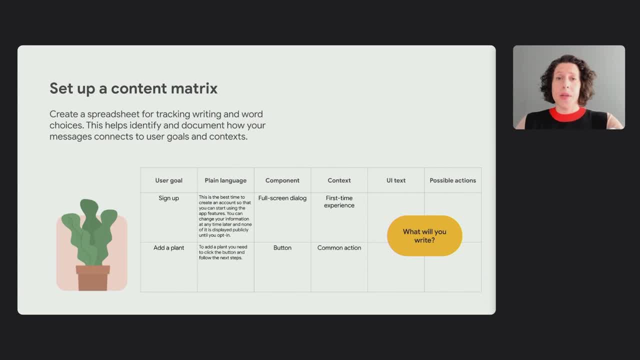 So if you've already defined the activity that someone does in soil and water as gardening, maybe calling it planting or hanging out in the backyard is going to start getting confusing. So I'll give you a minute to look through what's in this table. 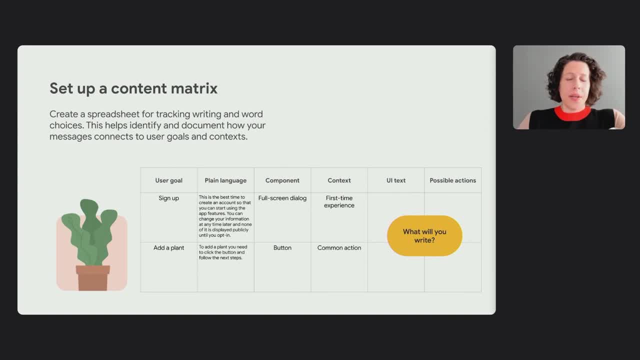 It starts with a user goal. You might already know these for your app or for soil and water. Of course, I made them up: Sign up, Add a plant. These are key actions. Then, in the next column, I think it's really important to try and state in plain language: 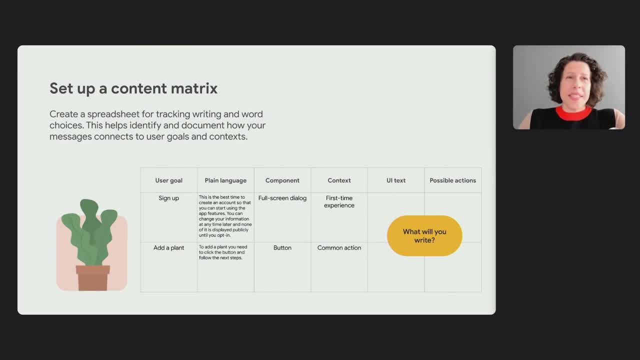 what you would want someone to do or not. And this is a key step to trying to go from your intention to what the UI text says. It's kind of an intermediate stage that will help take you into the most succinct and clear expression of the idea. 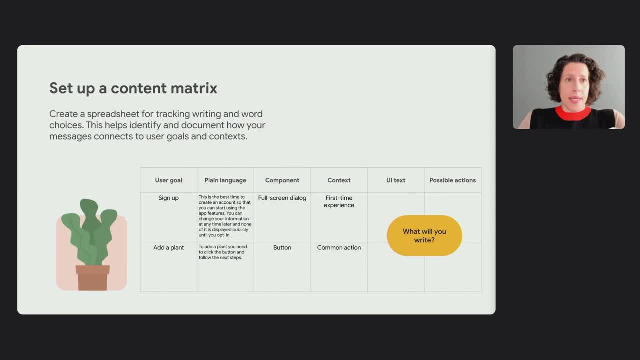 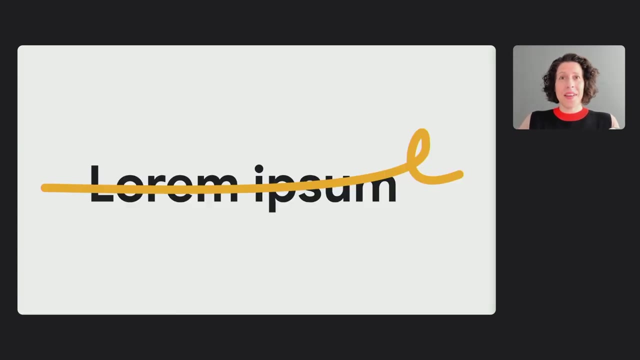 After the plain language, where you really get down, what is the core idea? here? I have a column for component Context And then UI text and possible actions. That's a key step. That's up to you. So what will you write there? 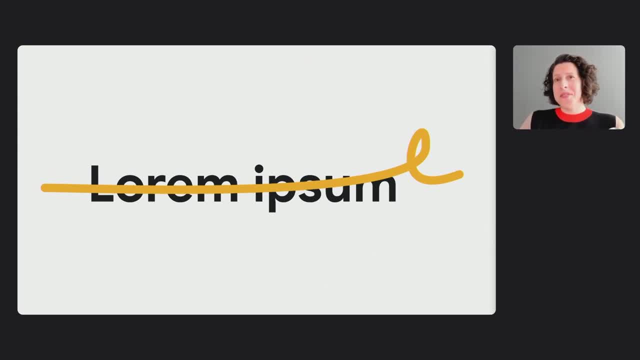 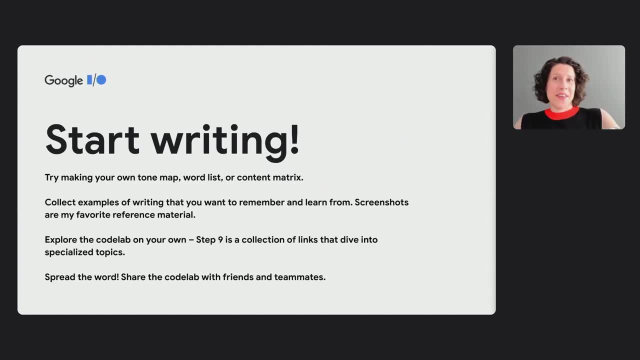 And so I hope, through a few of those steps, you have thought of a few new options and ways to approach an empty UI. You're on your way now, And getting better is in your hands, So I hope you try making your own tone map, word list, content matrix. 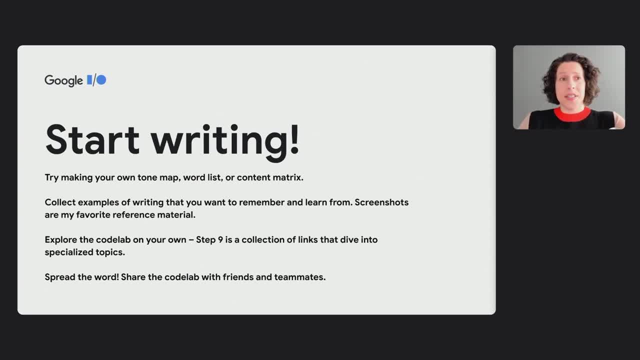 Another tip that I really like is I'm always taking screenshots for reference material of my own. You know UI text is out in the wild And it's fun to remember and think about it. So if you go back to the code lab on your own, step 9 also has a collection of links. 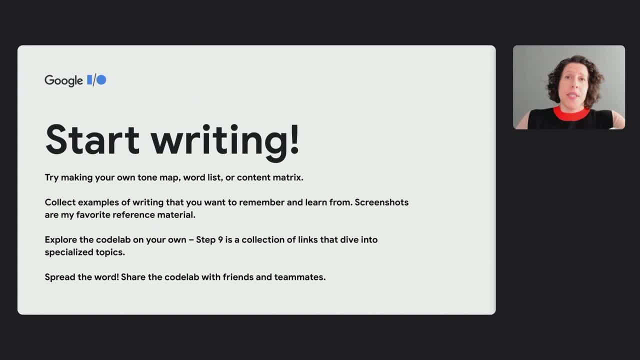 that dive into specialized topics. Some of those I want to mention are how to write for global audiences. It's a Medium article actually. I really recommend it. The other one I mentioned is accessibility labels and alt text. Google also has a great resource for conversation design. 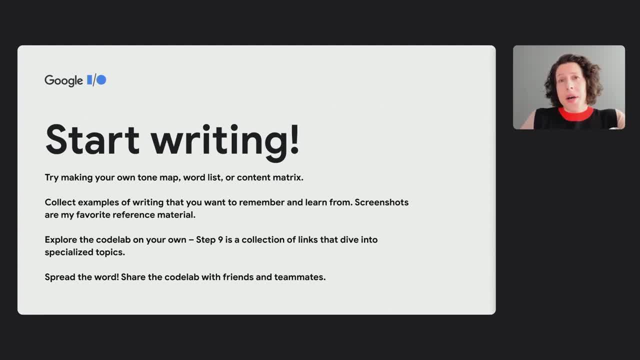 And actions on Google Assistant And the Android auto messaging for driving context is also a wonderful place to start thinking about that user context. Finally, you might have seen this at IO in 2019.. There's a writing for machine learning features section in the pair guidebook. 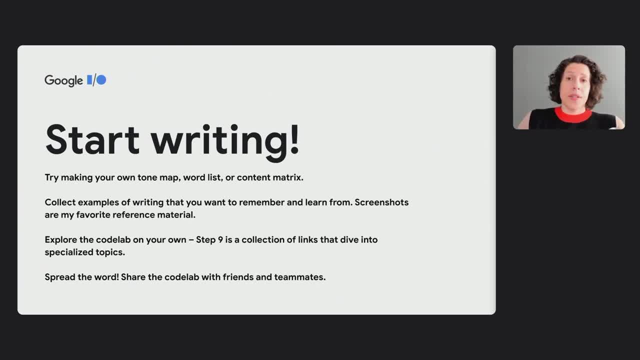 Thinking about how people get introduced to machine learning features is a really exciting thing to think through And has a lot of unique user needs- User needs around explaining what's going on behind the scenes. So if any of that appeals to you or is involved in the work you do, I highly recommend step. 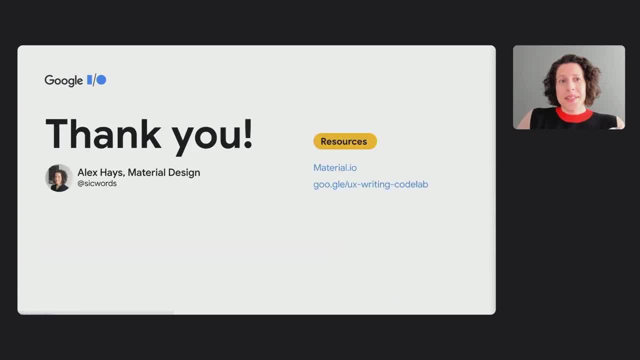 9 in the code lab. So I think we have time for a few questions now. Let me check the Dory. Thank you everyone. Here are the resources for material And this is the link again for the code lab. Okay, 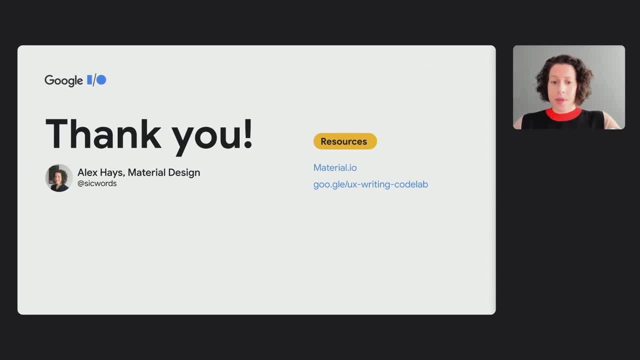 What questions are out there? Bear with me one moment. I'm going to the virtual Q&A, All right? So there's a great question about: do I recommend using emoji in a UI? Yeah, So, even in UX writing, the question of how symbols make their way. 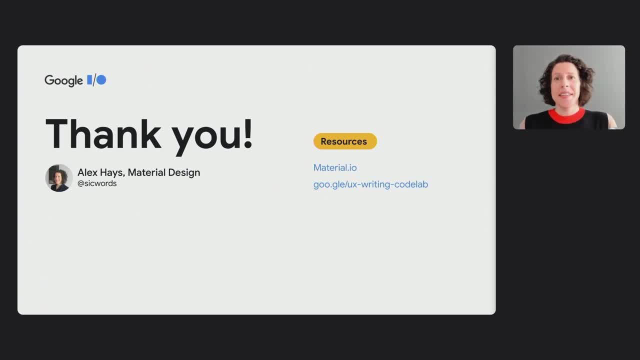 And combined with text is really interesting. I think that symbols, icons, communicative elements. they're really popular right now, Especially in social communication, And it started in the 80s with Kaomoji in Japan And Carnegie Mellon on the list. serves with emoticon, the colon and the parentheses. 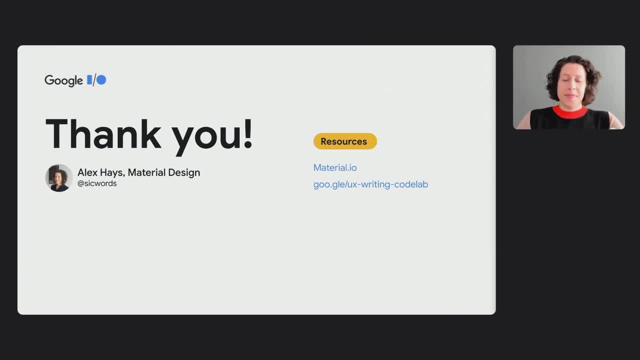 And I really recommend Gretchen McCullough's book Because Internet It's a book on Internet linguistics. It really dives into the nuances of emoji, So they're standing in a lot of time for emotion and prosody, The way people speak. 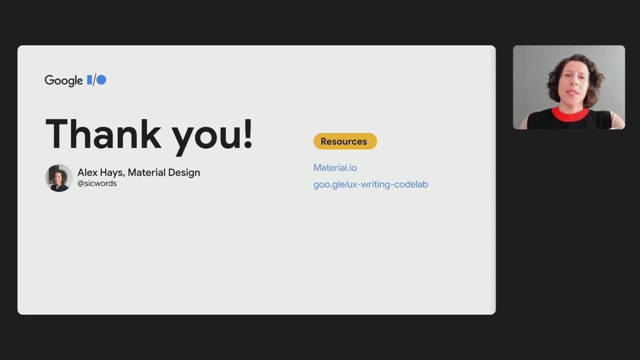 And they mean different things to different people. So if you go back to the goal of UX writing and that's to help people get through a task, to be goal oriented, you have to think in that moment, would an emoji help or hurt? 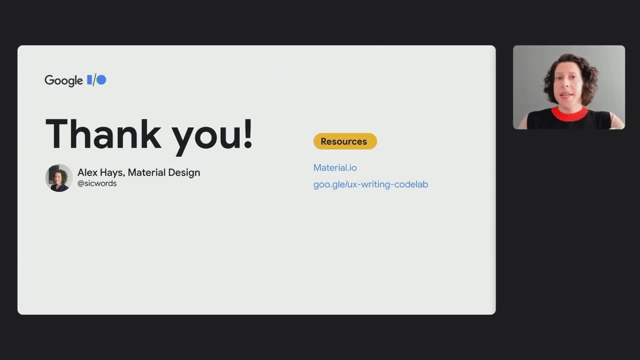 Is it there just for fun? Will your users understand it? Anything could also really help get those answers instead of just trying to guess, And the other thing to consider is that they can mean different things to different people. A lot of those gestures that we find in our keyboard, they're not universal. 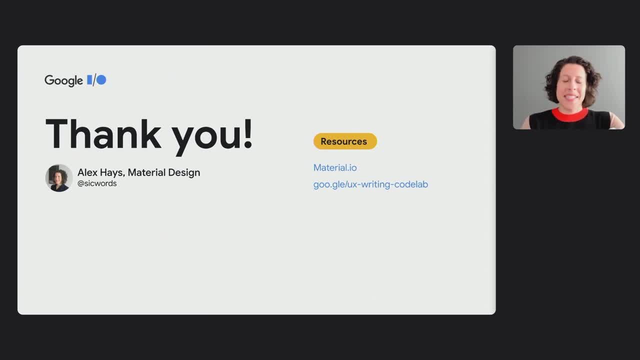 So my short advice is to use care, Because symbols are not universal And neither is language. So I hope that answers the question about emoji. I hope we can add some emoji writing guidance into the material specs soon as well. I think that would be really helpful. 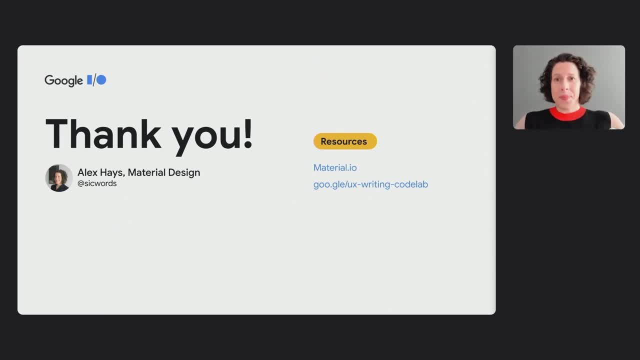 Because not all emoji are created equal, actually. Okay. Next question, Let me check this out. Okay, What about tools that use machine learning, Like Gmail's Smart Compose? Okay, That's a great question. That's the question that cuts right to the core of: will I have a job in a few years? 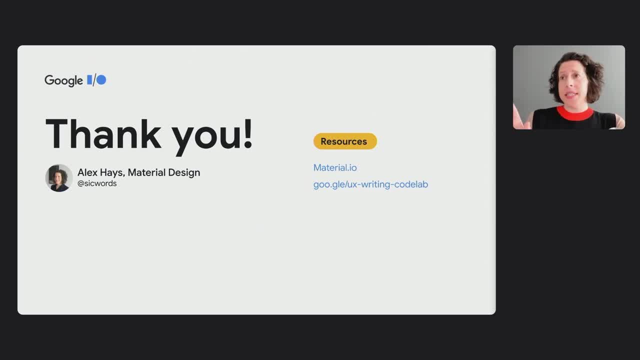 Gmail's Smart Compose is amazing. It anticipates the rest of your sentence. It's built on a corpus, I believe from using Reddit user's threads, And for me personally it anticipates my thoughts really well, So I use it often. 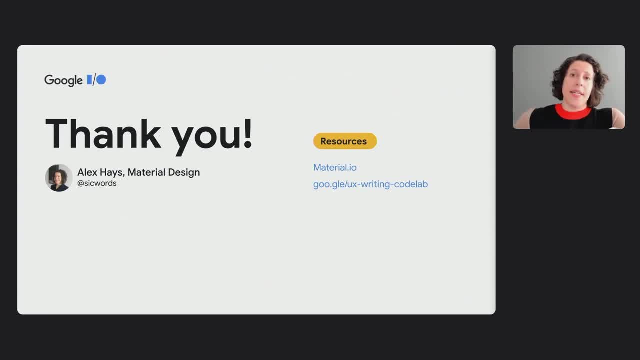 I think it's helpful Write AI writing. Okay, It's a tool, It's a kind of cooperative, collaborative communication between computers and humans. these days, It's a lot more than just AutoCorrect. now, And in the case with Smart Compose, people think that writing emails daily is tedious. 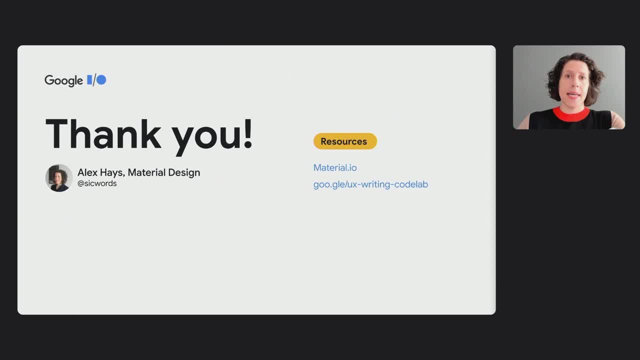 You write the same thing over and over again And can save a lot of time on tasks through this, And that's definitely true. Issues of like representation- Yeah Yeah, representation in the machine learning- have also come up in the way that the word like doctor. 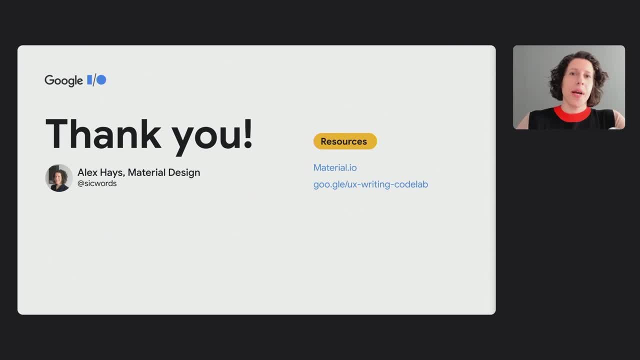 might always trigger a male gender pronoun to follow. So there's a lot of challenges there, but it's also- I've also seen it described as well- as a question of equity. Language can be a barrier in the workplace, especially in the norms of a non-native language can be very hard. 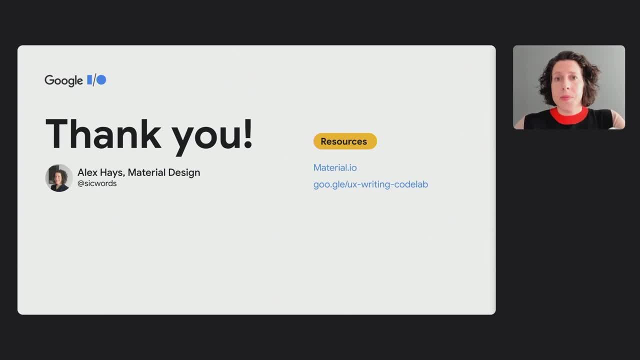 professionally, So this makes a lot of people's experience smoother. So, that said, I will say that I'm also a firm believer that writing- whether it's an email or in a doc, or for your own products- I would say it's a way of thinking. Writing is thinking, So if you don't really go, 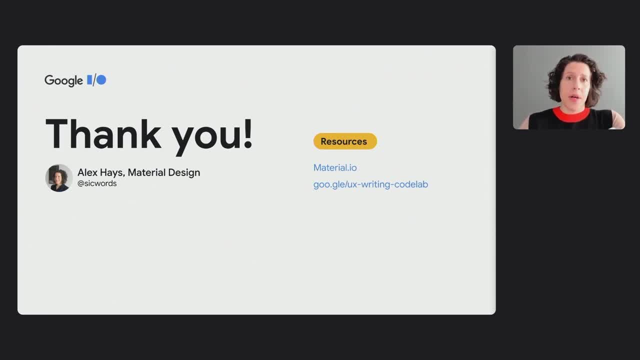 through your word choice and revise, you miss out a lot on what writing has to offer. I think that going through and revising is really where a lot of the improvement happens- in writing too, So there's some amazing tools out there I think you can use. 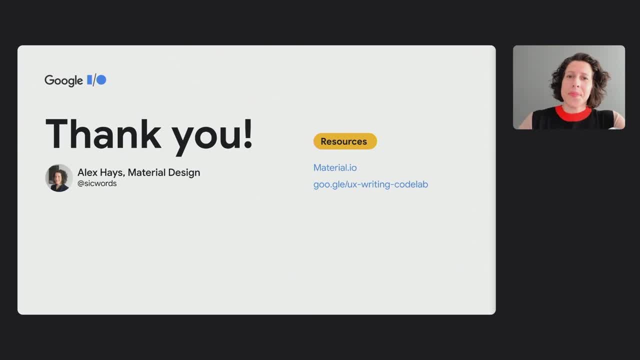 them in combination with what you're trying to achieve. All right, I think we have time for a couple more questions. Let me check the forum And a quick shout out to my teammates Louise, Ivy and Megan, who are helping answer some of the questions. 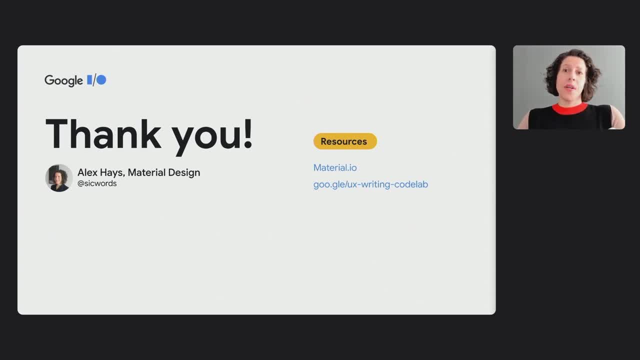 It'll be open for 12 more hours after the talk is over And I'll jump in And you can also feel free to find me on Twitter. Very new, I'm not very good at it, But I'm excited to connect with the developer community, So send me any questions you have. 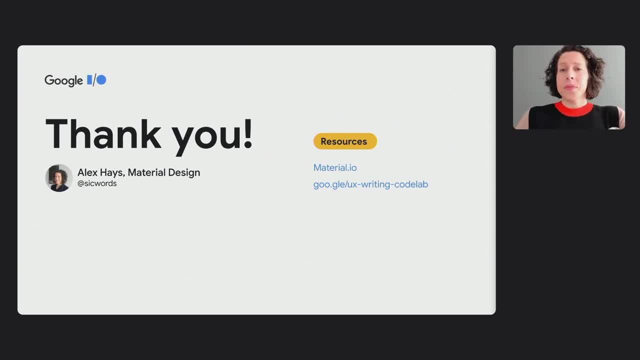 All right. So one question I have is short sentences sometimes use imperative language. For certain usages, like talking to kids, it might be perceived as aggressive. How do you suggest that's balanced? Okay, So imperative language. You see that in some of the examples I gave around buttons. 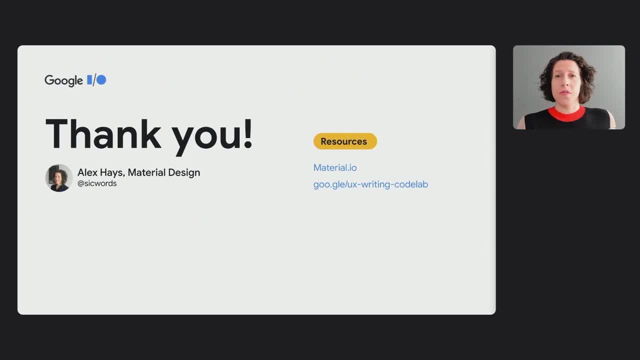 Add plant is also a little bit of a little forceful. It's very direct When you talk to kids or a lot of other scenarios. it's not good to be quite so commanding I think. So I would say it's not just kids necessarily. 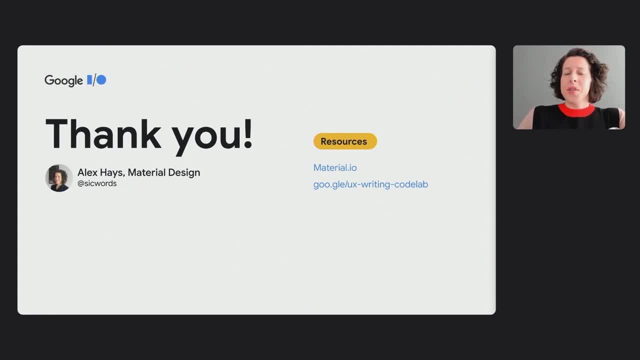 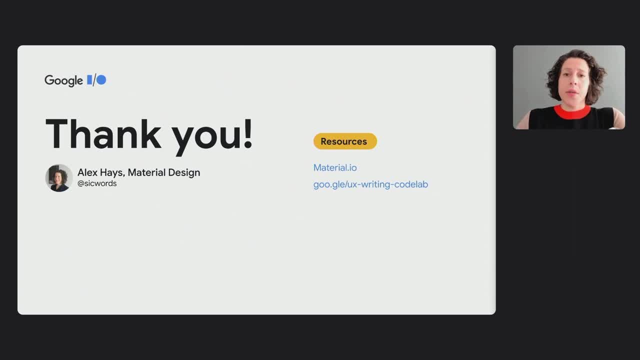 the way you phrase things in those contexts are really consequential. Okay, Another question is: when would you recommend using an icon versus text, For example, inbox icon versus the word inbox on a button? Well, I would recommend using both of them most of the time. 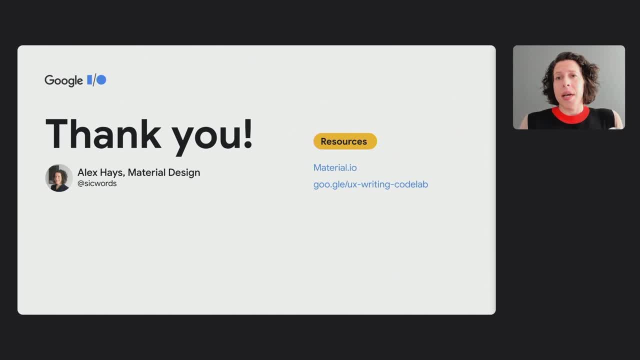 Screen space is tight, of course, but labeling your icons with text is a really important measure to make sure that your work is accessible. So assuming that the icon's meaning is universally understood is just not as inclusive as it could be. So 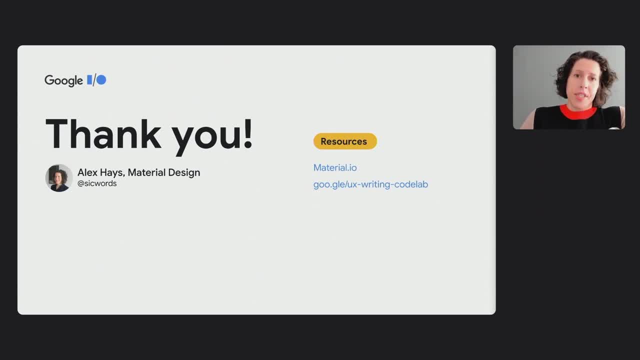 the word inbox on a button makes sure that more people can get the most out of an experience. Another thing people do is hover states, So a tool tip would have that label contained. It wouldn't always be visible, but it's available on hover. You say that around a lot in a lot of. 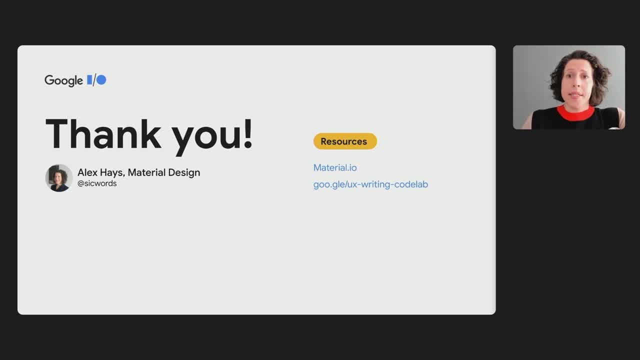 symbols in Gmail for other tools And that is an interesting way of handling like a contextual need that you don't expect someone to learn but want them to have often. So in general, I think screen spaces are tight. Bottom navigation leaves so few.